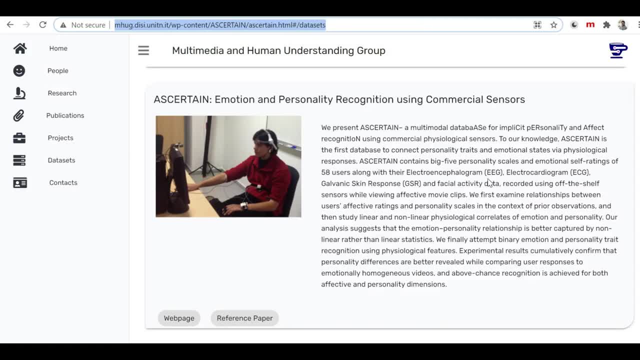 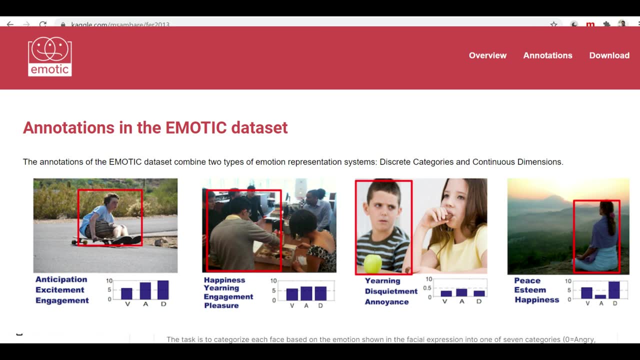 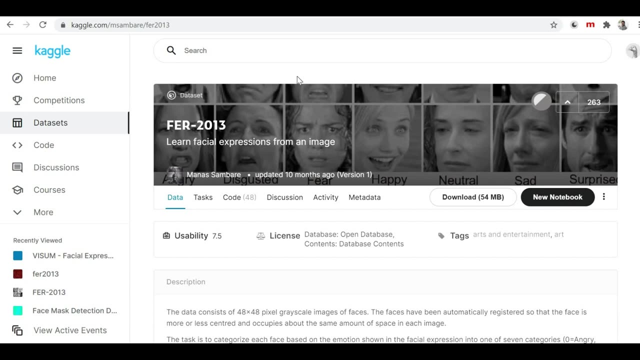 you can go and see the different kind of readings made with the different sensors at the particular, different type of situation and based on that, you can do the emotion detection. But in this episode I am going to make use of FER 2013 facial expression data set for doing the emotion detection, So I will provide the link of this. 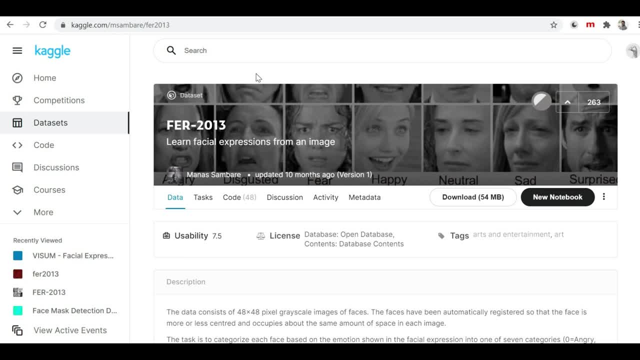 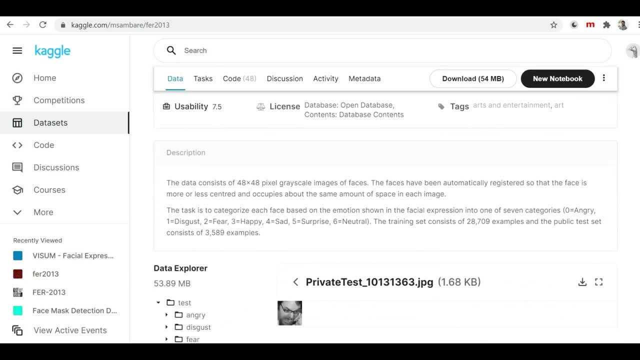 data set in the description box. so if this data set is available on the Kaggle platform, you can easily access it and download at a free of cost on your computer system. So you can get the more details about this data set, like here it having the 48 by 48 pixel grayscale images of the faces. 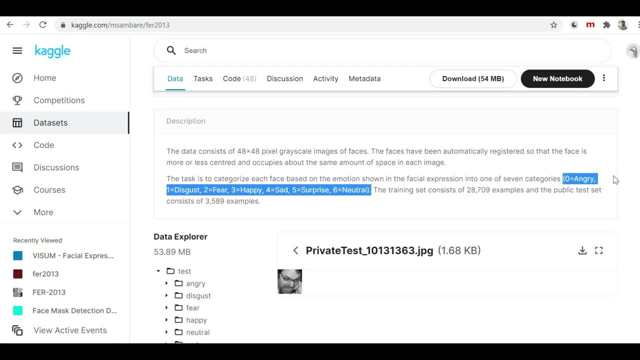 and it contains the different seven categories of emotions like angry, disgust, fear, happy, sad, surprise and neutral. So on this data set we have around 28709 images for the training set and in the test set we have around 3589 images. Ok, so this is the good amount of data set to develop any. 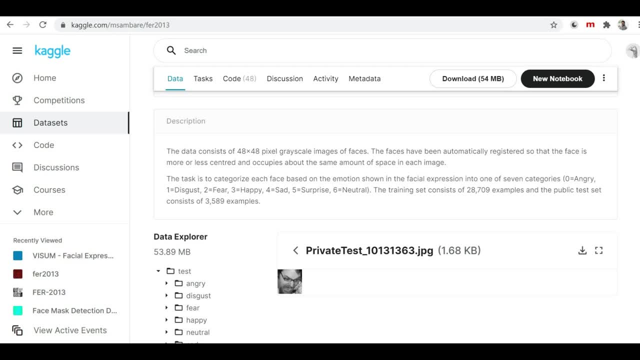 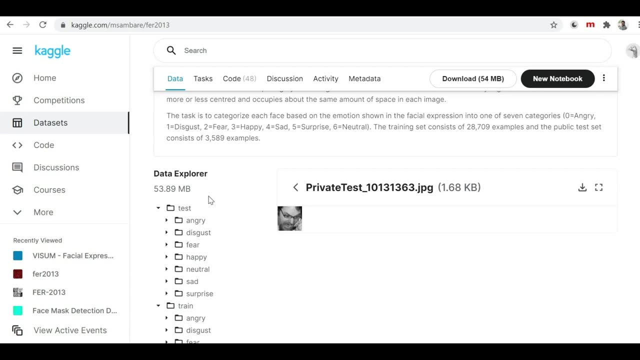 emotion detection system at a beginner level. Ok, so the overall size of this data set is 53.89 mb, because these all images are small size of 48 by 48 pixel and all images comes in the grayscale. So inside of this data set you will be able to see that this image is contraindicated. The image is: 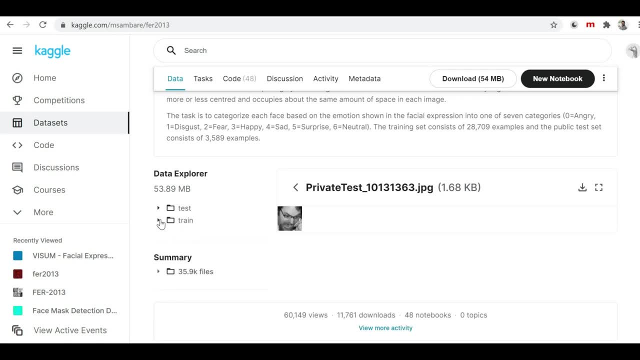 this data set. you will find that it having the test and train folder, so i'll explain all the folder structure in the our pycharm id. so let me just quickly go and download this data set. so if you want to download, you can click on this download button and it will download this data set on your. 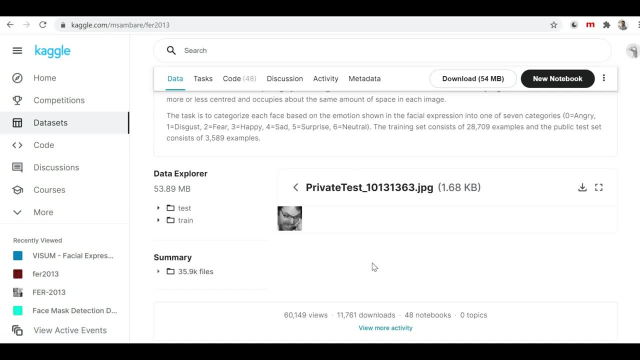 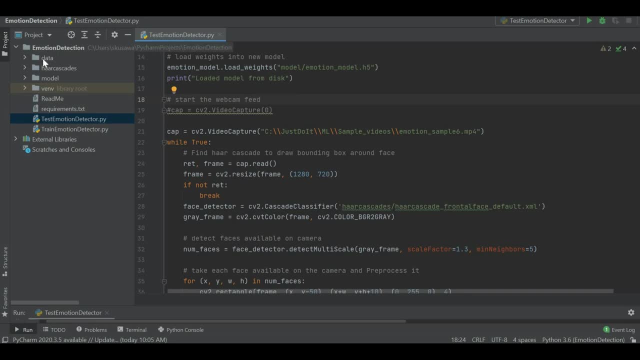 system. so i have already downloaded it and added inside of my project. so let me jump back to my pycharm id. so here you can see that inside of my emotion detection project here i'm having one folder data. so this is the folder i have downloaded from a caggle. so just now i've shown you the f. 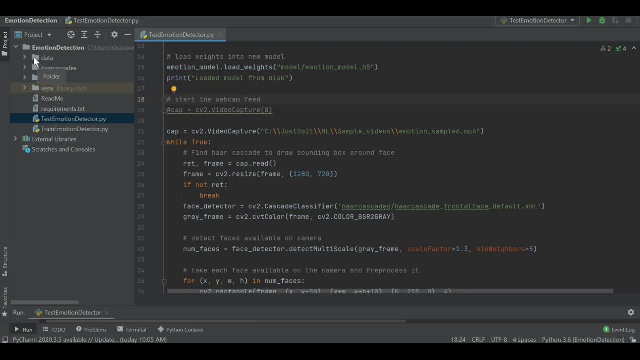 year 2013 facial expression data set. so that same data set i have kept inside of this data folder. so if i just open this data set folder, i'm having my train data and test data. okay, so these are all the two folder. if i just open this train folder, i'll find the seven other folders, which are: 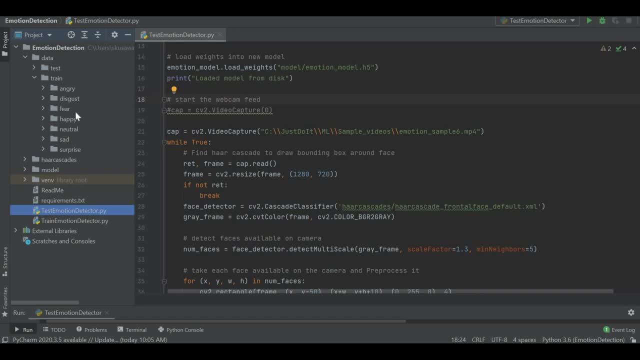 representing the different emotions like angry, disgust, fear, happy, neutral, sad and surprise. you can see that i have downloaded this data set. so if i just open this data set i'm having my train data, and if i just go inside of any of this folder i'll find the plenty of images. if i just 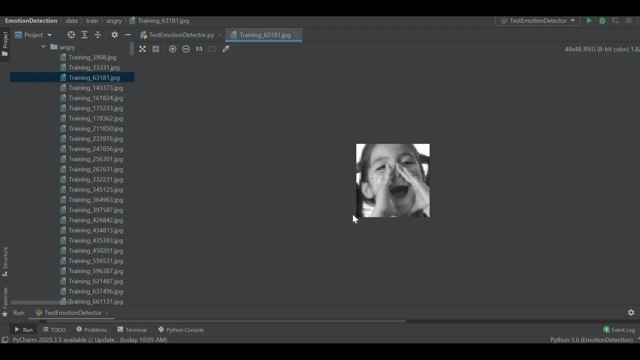 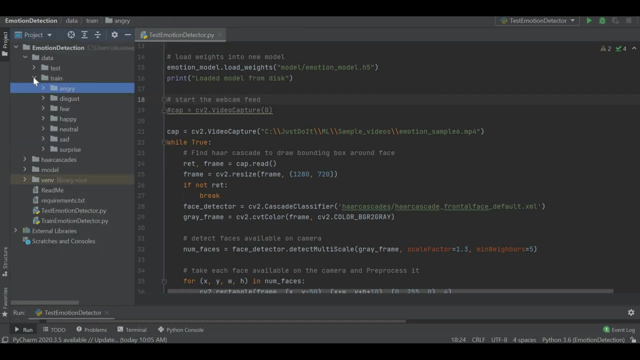 try to open it, you can see that we have the 48 by 48 pixel grayscale images. so these are all the images related to the angry emotion. okay, so, similar way, i'm having the plenty of images related to the each emotion in this, each of this folder. okay, so let me just collapse this train. 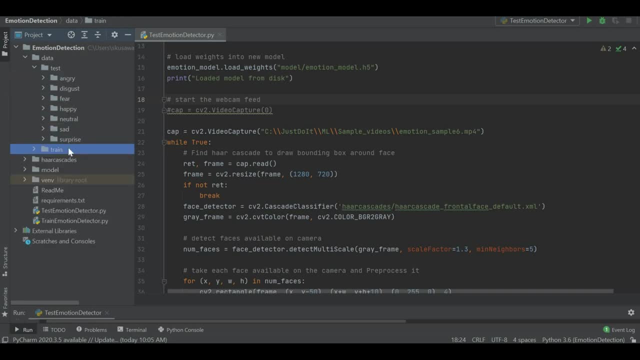 folder and similar way inside of test folder. i'm having the seven emotion folders and respective images inside of this. okay, so now i have downloaded and kept my data set inside of my project directory. so in this project, first of all we are going to design our own convocational neural network and after that we 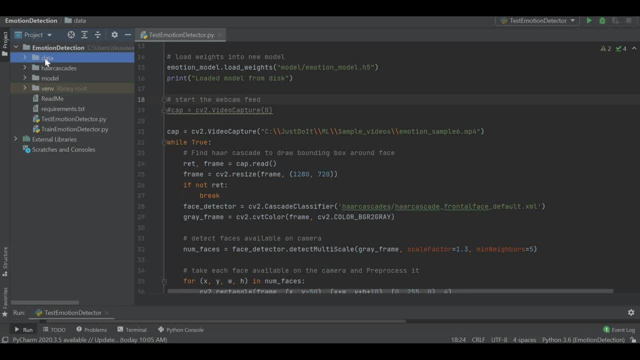 are going to make use of this data set to train our neural network and once it trained, then we are going to make it use for the prediction purpose. okay, so now let me quickly show you that which are all files we have. so one file we have for training our emotion detection model. so 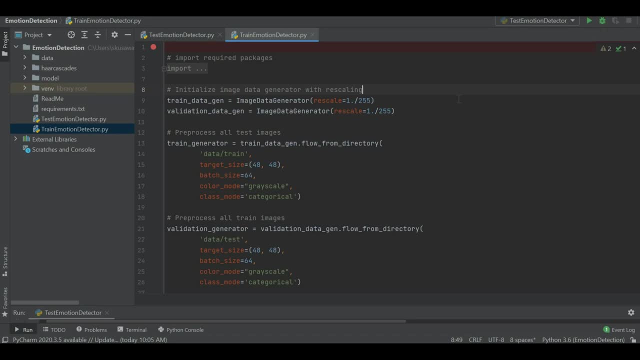 this is the file which we are going to use to train our emotion detection model and this is the motion detector. i'm going to explain all this code line by line in couple of minutes. okay, so this is our second file, test emotion detectorpy. so this file we are going to make use for. 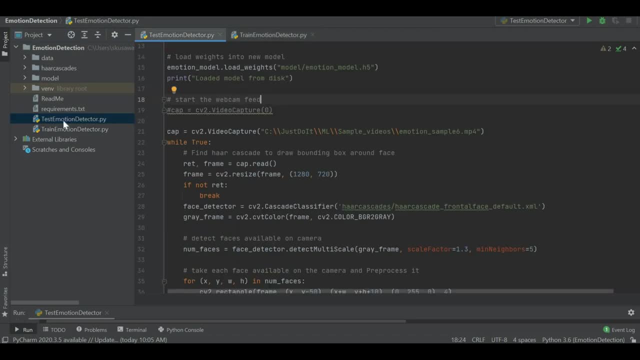 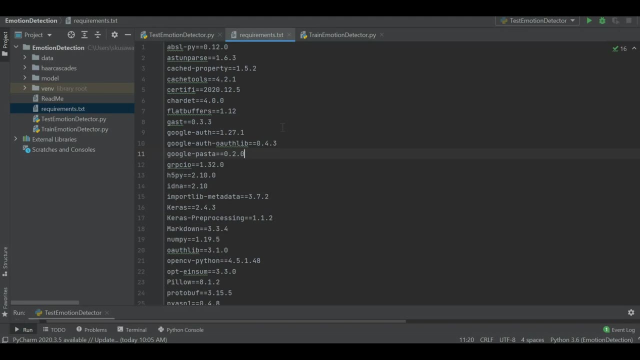 actually doing the emotion detection on the video as well as in the real time by using our live feeds of a laptop's camera. okay, and this is the requirementtxt file, which contains the all the libraries i have been used in this project. okay, so you can see the plenty of libraries, but actually, 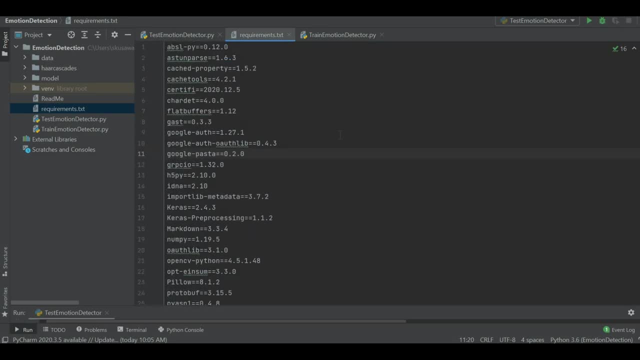 i have installed a couple of libraries and those libraries having the odd dependency on all the other libraries, so you can see the there are plenty of libraries, so you don't need to worry about. i'm going to provide this all code on the github repository you can access from there and 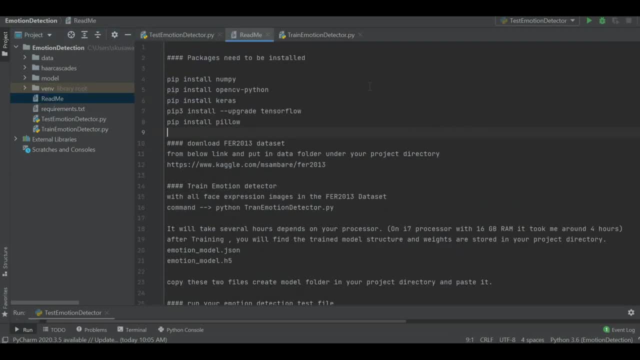 i also provided the readme file over there so you can see that this is the readme file. you can follow this file. you will know that, which are all packages you have to install, how to download the data set and what are all steps you have to follow to run this code. okay, now let's come back to our 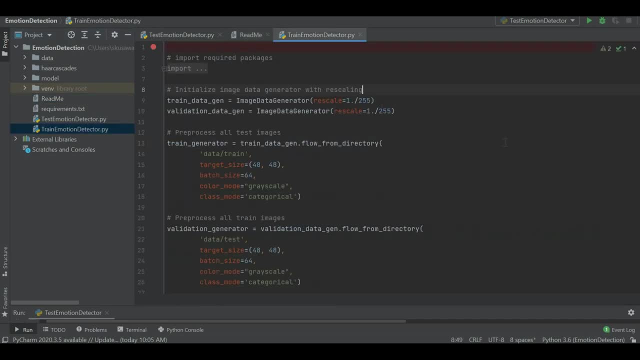 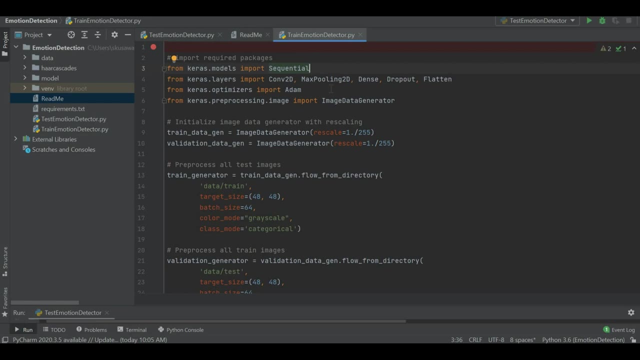 train emotion dot detector file and let's try to understand that. what code we are going to use for training our emotion detection model. okay, so first of all we have to import the all the packages required for training our emotion detection model. okay, so it will contain the all the modules which 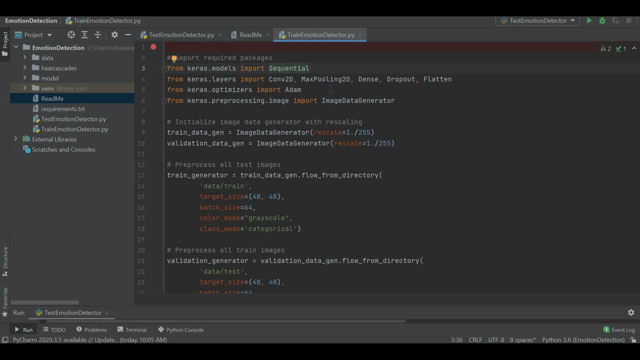 we need to develop our convocational neural network and there are a couple of classes or modules. we need to pre-process our all images before passing it for the training to our convocational neural network. these are all the packages i have imported from the keras library. 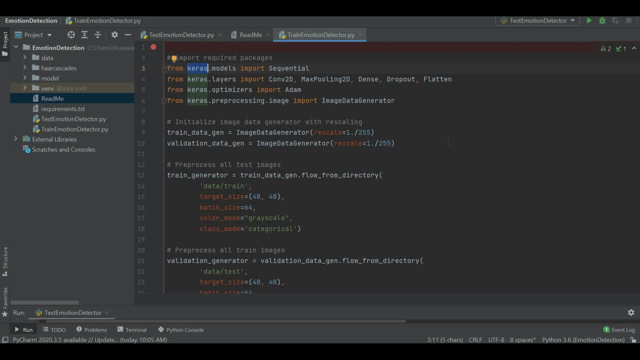 okay, and this keras in the back end uses the tensorflow. here you can see that i am generating the two image data generators. so these image generators i will be using for pre-processing my all the images. so whatever the images we have inside our facial expression data set, so test and train images, we are going to pre-process these all. 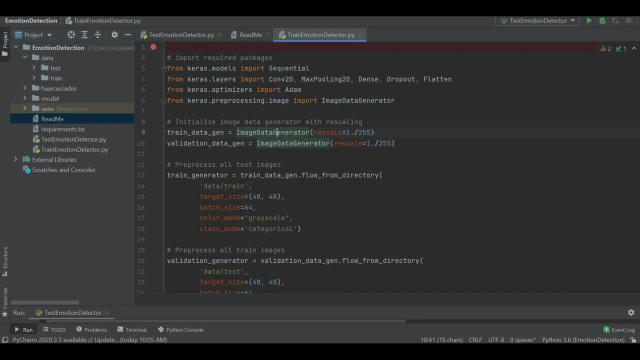 images. so i have created the two image data generators, one for the training purpose and one for the testing purpose, or you can say the validation purpose. so here you can see that i have accessed the train data generator and i'm you making use of flow from directory. 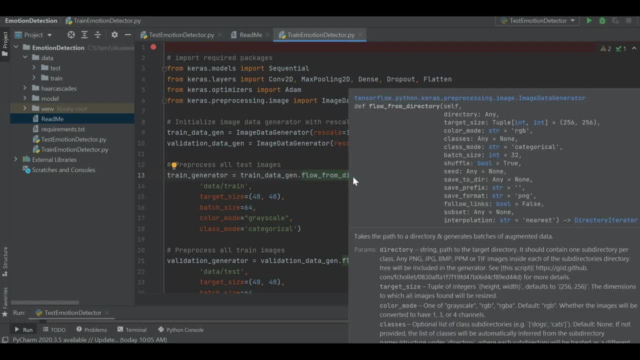 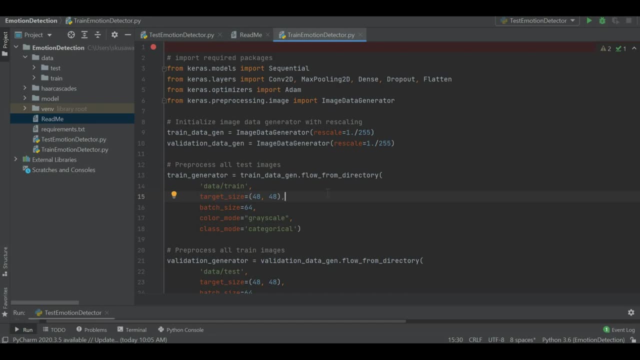 okay, so this flow from directory is a very good tool in the keras where you can make use of it to just flow through the directories and collect all the datas and pre-process it. okay, so what it will do, i'm just passing my train directory. okay, so inside of this, you can see that, inside of data. 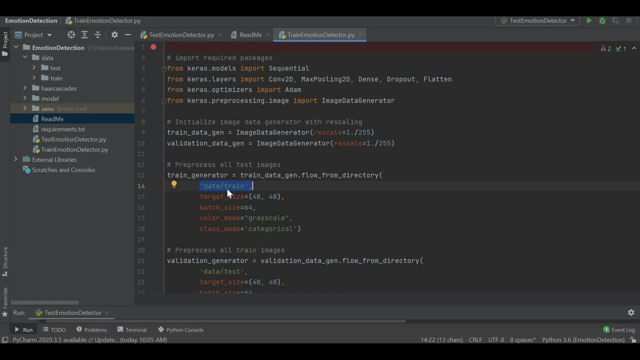 i'm having the train folder so i'm here passing my path like data slash train. so it will go inside of this train directory and it will collect the all the folders and go inside of all the folders and it will fetch the all the images and whatever images you have inside the train folder you can. 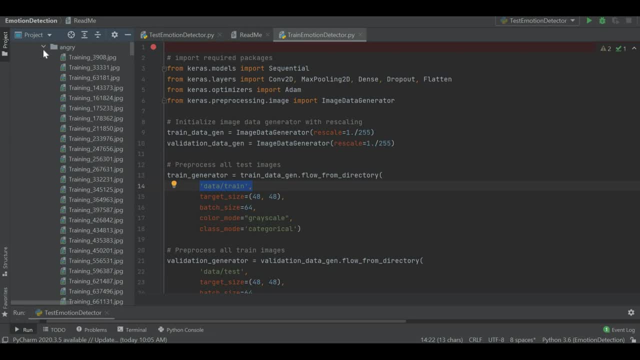 also see that it will label the images you have inside the train folder and it will label those all images with label like angry and similar process. it will do with all the rest folders. okay, so here i'm providing our target folder and here i'm providing the target size, so each 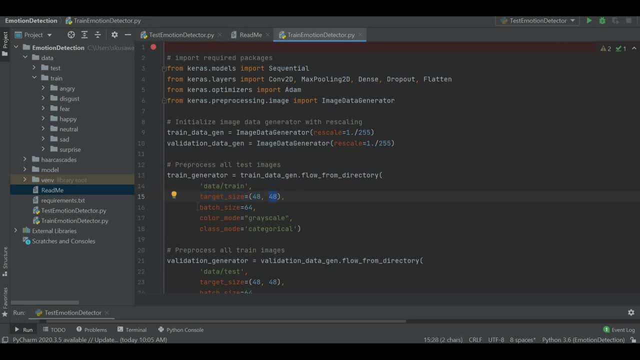 image will be resized to 48 by 48 and it will do in a batch size of a 64 and color mode will be gray scale. okay, so whatever images we are loading, it will be in the gray scale and the class mode will be the categorical. see means that whatever the folder structure we have provided, 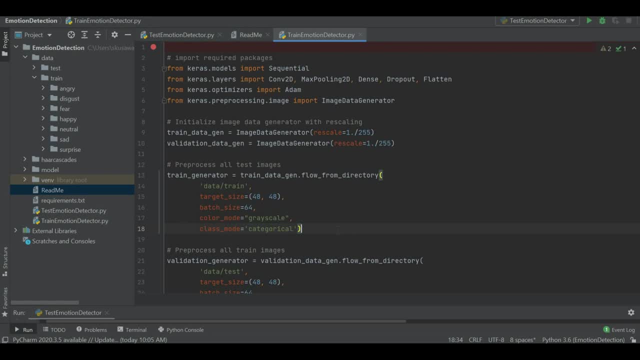 according to that, it will create a categories. okay, so this is a very easy and handy tool. i frequently use this tool when i use the folder based image data. okay, so here you can see that. similar way, i am creating the our validation generator. again, i am flowing from the directory. 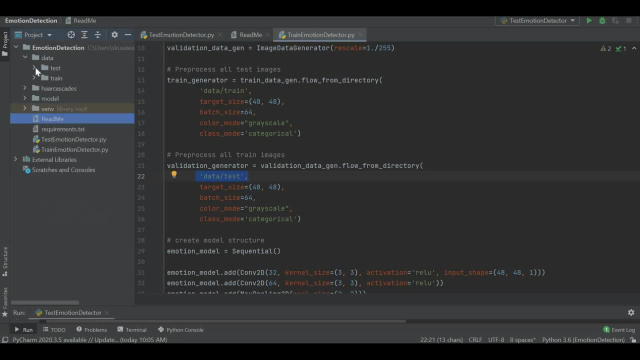 passing our text directory. so let me just close train one and you can see that test directory. it is having the similar kind of folder and i am passing the similar configuration like target size is 48 by 48 pixel, bath size, 64, color, grayscale and class mode as a categorical okay. 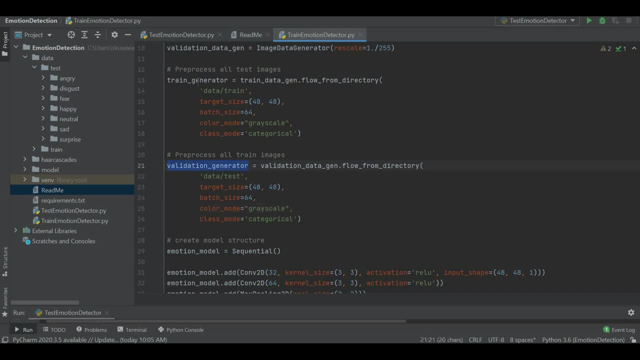 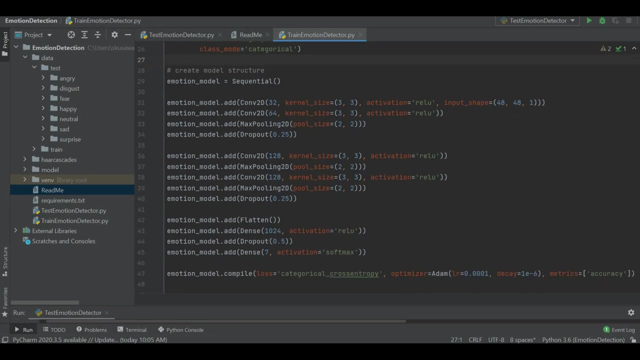 so now our both generators are ready: train generator and well data generators. it means that our all the training and validation data is now pre-processed. okay, so now let me just move next and create our convolutional neural network. so here you can see that one big size of. 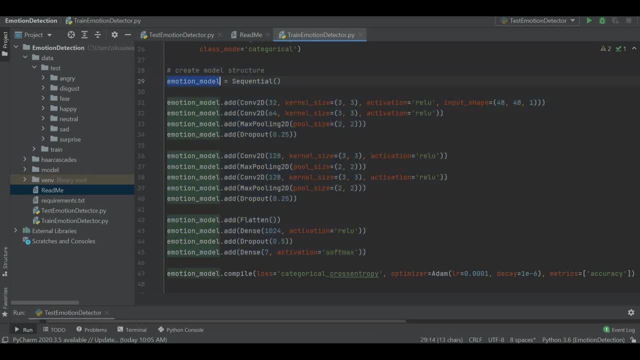 convolutional neural network. so from keras i am just accessing the sequential neural network and i am just accessing the sequential neural network and i am just accessing the sequential model and inside of that i am adding the different layers. so you can see that i'm here adding the convolutional 2d layer with a 32 size and kernel size is a 3 by 3. 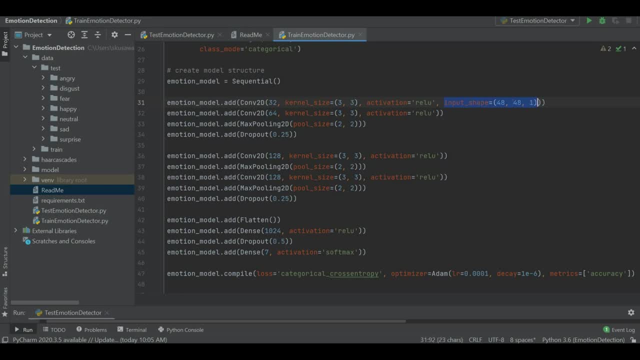 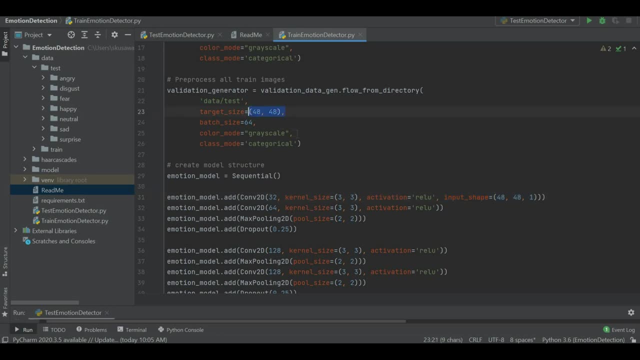 activation function is a relu and the input shape means that whatever the images we are passing, so just we have all the images pre-processed with a 48 by 48 size and color code is a grayscale. it means it is having the only one color channel. so here i am passing the input shape as a 48 by 48. 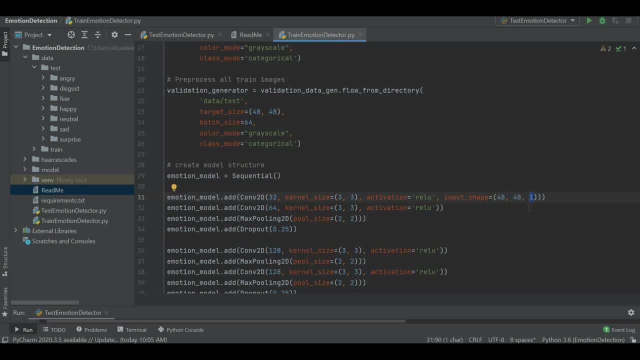 pixel and color is only one gray scale and we are passing the images with a 48 by 48 pixel and color grayscale, so i'm passing the color channel as a one. if it is a rgb image then we have to pass it like a three, but most probably we don't use the color images for training models because it takes 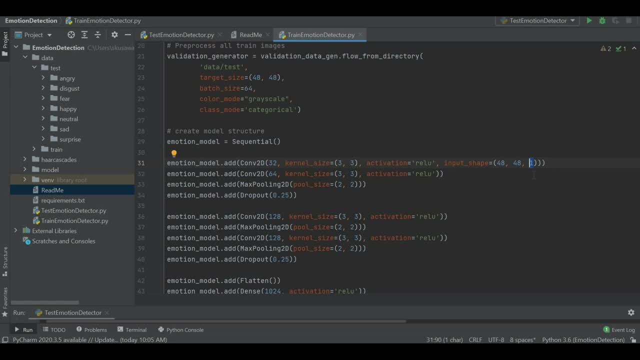 a lot of time. so we need that powerful systems so we can go with the more channels. okay, now let's coming back to here. again, i'm adding the another convolutional layer and with a 64 size kernel, of same three by three, and activation function is a relu. and then i'm going to add the pulling of. 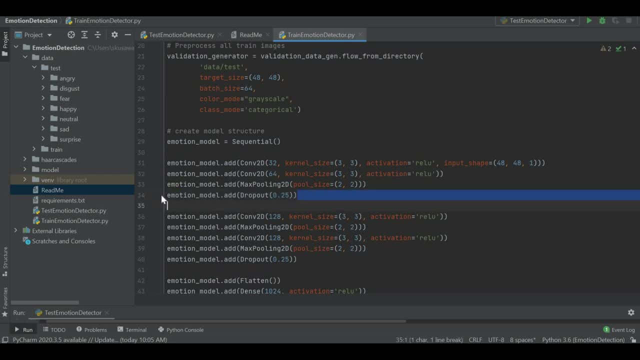 two by two, and to avoid the overfitting, i'm just going to do the dropout with 0.25. okay, so similar way, i'm just adding the another convolutional layer and the pulling layer and again i'm adding the convolutional layer and pulling layer and just to avoid the overfitting, i'm again doing the. 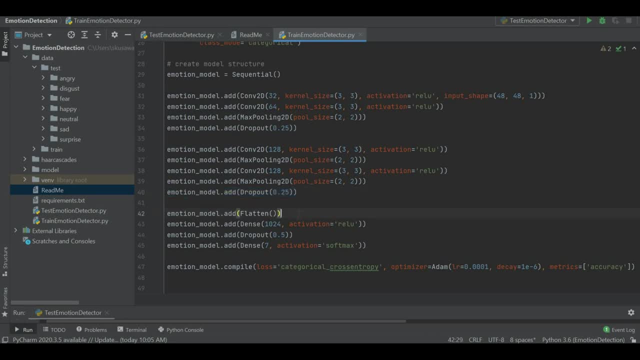 dropout of 0.25. and here you can see that i'm just adding one flattened layer to flat the all the values and after that i'm again applying the dense of the 1025 and the dropout of 0.5 and at the end 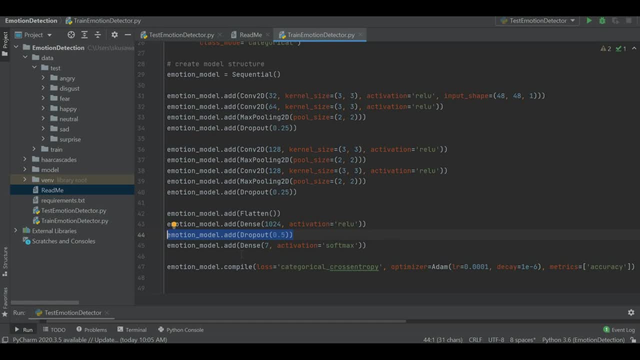 we are going to get the seven r classifications or the categories. so i'm here adding the last dense layer with the seven categories. so these are nothing but the r7 emotions and i'm adding the activation function as a softmax. okay, so this is the r complete convolutional network. and now. 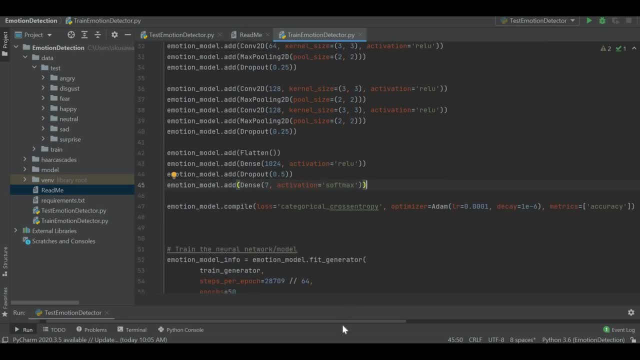 i'm going to compile this convolutional layer with a loss function optimizer and are the metrics for this particular model? okay, so here you can see that i'm adding the loss function as a categorical cross entropy, i'm adding the optimizer as an atom optimizer and with learning rate of 0.0001 And DK of 1 e raised to. 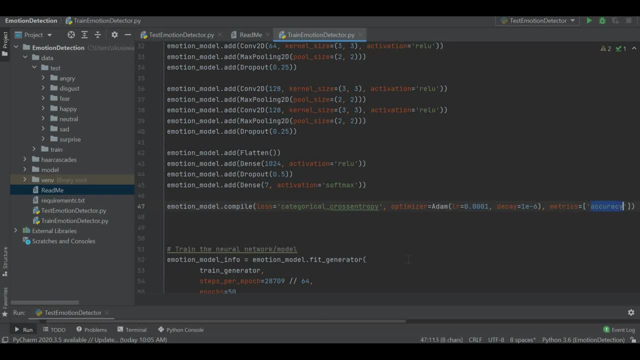 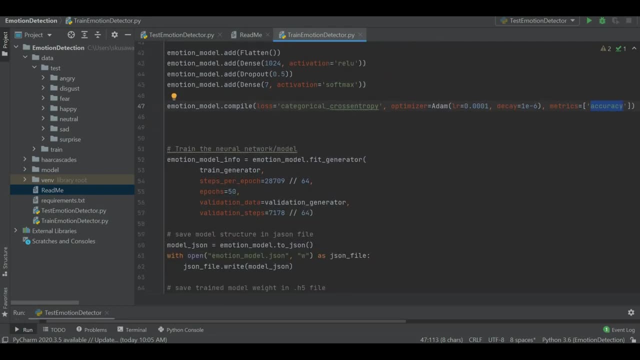 minus 6. okay, and i'm using metrics as a accuracy. okay, Now our model is ready and we have chosen our last function: optimizes and matrix. Now we have to train: are this convocation neural network with our preprocess data. so here you can see that what are the emotion model we have just designed to this we are. 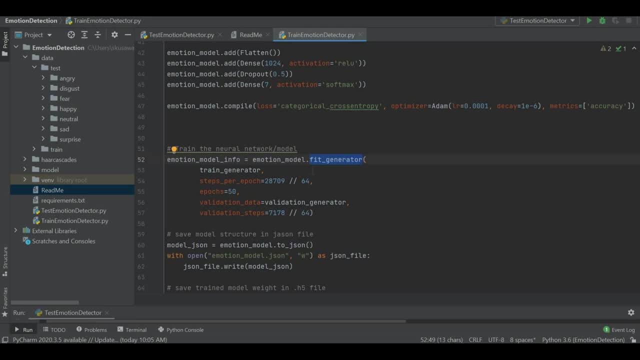 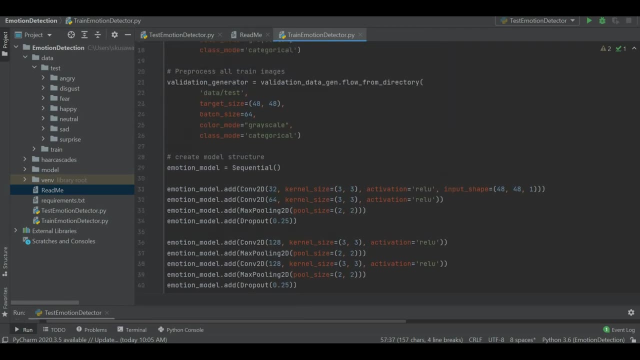 going to fit? are all the data okay? So this means that I are making use of feed generator, which will take the all the train generator data okay. so whatever data we have pre-processed, so here, if you go on the top, so we all the training data we have. 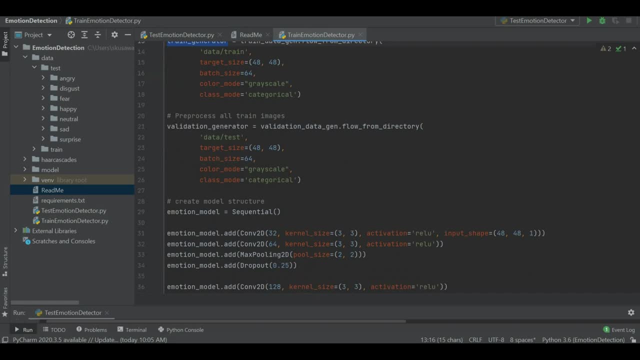 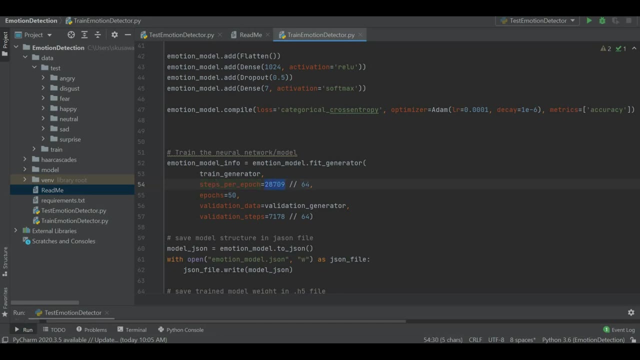 pre-processed and stored in this train generator. okay, so i am just going to pass this train generator over here. okay, and here i'm going to say that steps for epoch is a total number of images divided by 64, and this training will happen for the 50 epochs. okay, so if your system is too slow, 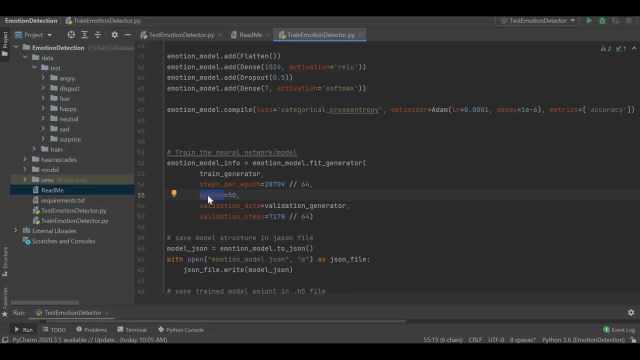 and taking too much time. then just try to reduce this epochs to 20, 30 and give a try. if you have a very good computational power, then you can go for more than 50 epochs. okay, but it will consume a lot of time, okay. so now here, validation data. i am providing validation generator, so this is the. 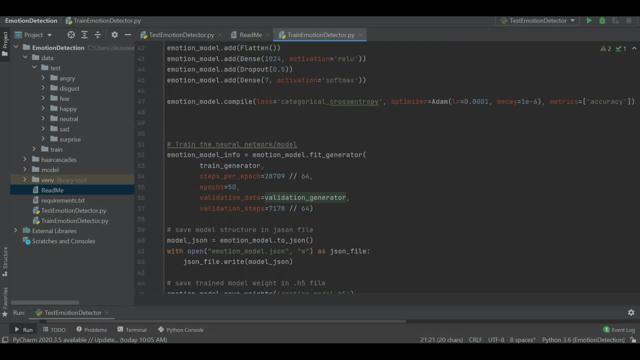 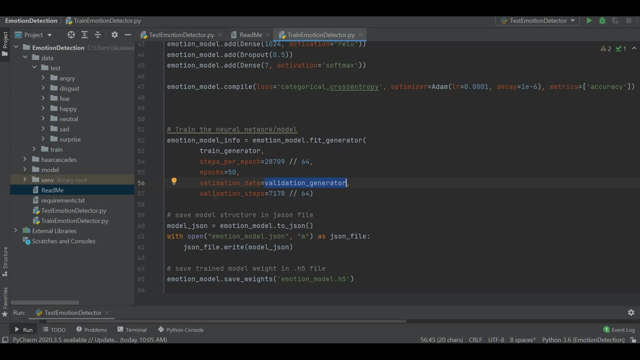 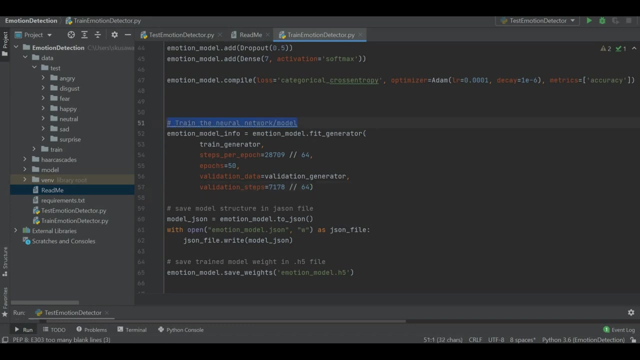 same data we just pre-processed. this is our validation generator. i am passing it while training our model or fitting our model, because it will evaluate that how well our model is working. and this is the validation step. so, total number of images divided by the 64.. at this step, our model will be get trained. our neural network will be get trained. 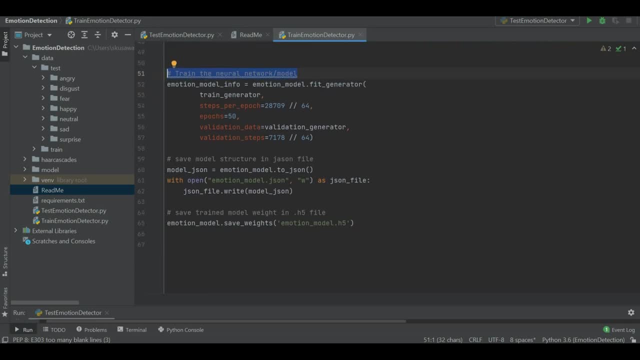 with whatever the data we have pre-processed now and it will also validate with the set of our validation data. so once our model is trained now we can store the structure of our model in the file, as well as the weights it learned from this- all the learning process, or the training process. 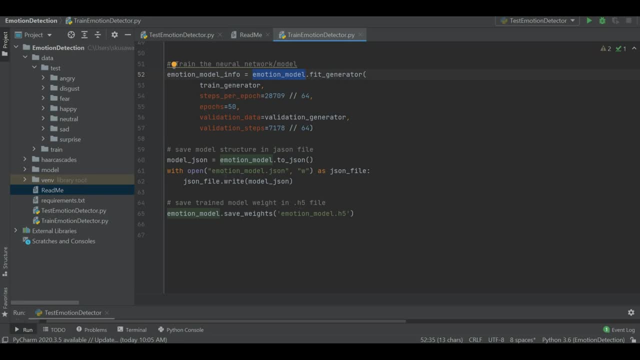 that we will store in the weight file. okay, so here you can see that i am storing the all the model structure in the emotion modeljson file and all the weights- learning weights- i am storing in the emotion underscore, modelh55. okay, so this file will be stored inside of your directly project directory. so it was stored in my emotion detection. 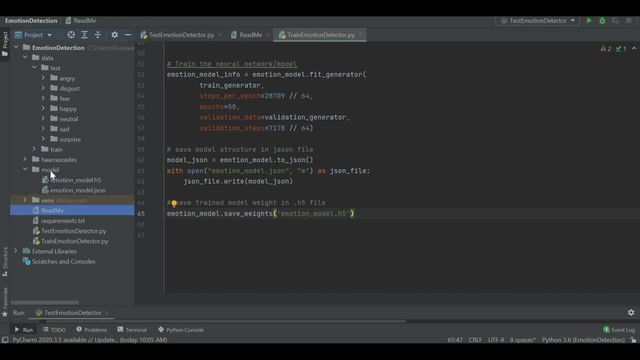 folder and from there i copied and i have pasted in this model folder. okay, so you can see over here. so i'm not going to train this model now, because it took around four hours for me on the i7 processor and the 16 gb ram. okay, so i was not using a gpu over here, i was just using a plain i7. 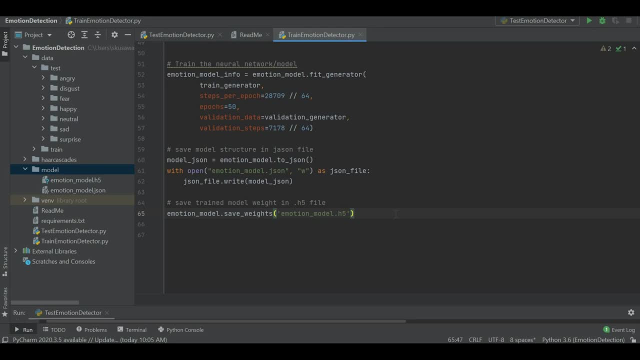 processor and the 16 gb ram, and it took me around four to four and a half hours to train this convocational neural network on this particular data set. okay, so, whatever data set i have trained, its weight and structure, i have stored in this model folder. okay, so you can see that this emotion. 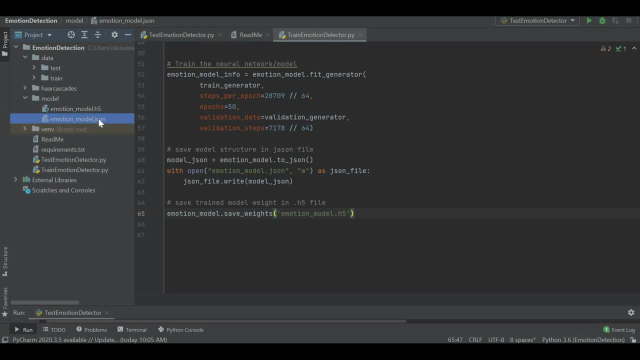 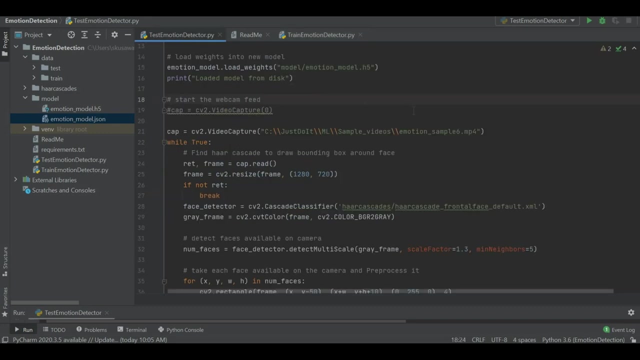 underscore- modelh5 and emotion underscore- modeljson file. okay, so now our training part is completed. now we have to go and we have to load this model and we have to apply on any video or live stream to check how it exactly works. so i'm just going to our test emotiondetectorpy file and now let's see that. what are all things we? 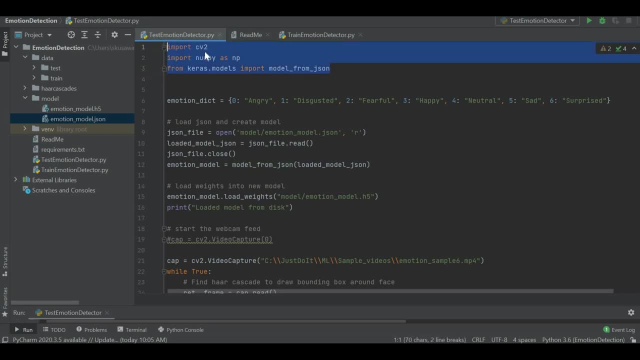 are doing here. so first of all i'm importing all these packages. opencv i'm using to access the live feeds from camera or to read the video content, and here i'm using a numpy to just numeric operation and this kerasmodels to load our model which we have just stored in this emotion modelsh5 file. 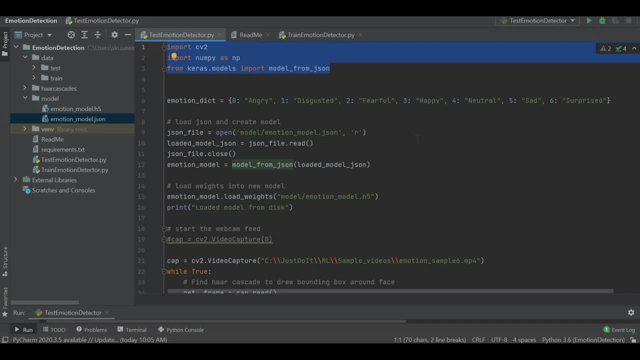 all the weights and emotion underscore modeljson. instead of that, we stored all the structure. okay, this is the list of. are all the emotions like angry, disgust, fearful, okay, so whatever the folder we had. so according to sequence, at the zeroth index we have the angry emotion, at a one disgusted. 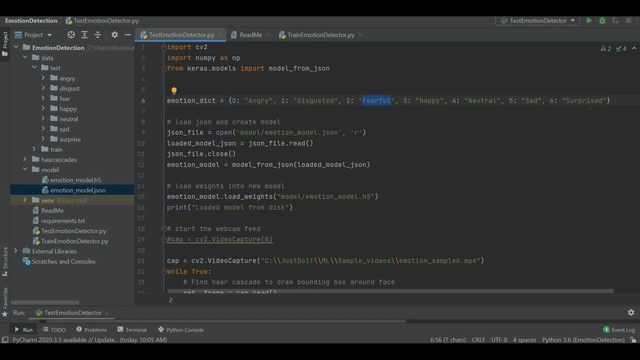 and two is fearful, three is happy, four is neutral, five is sad and six is surprised. okay, so i have just created the dictionary. so at the output, whatever the output we are getting, we can directly map with the label. okay, so if it is giving that emotion is a zero, it means that. 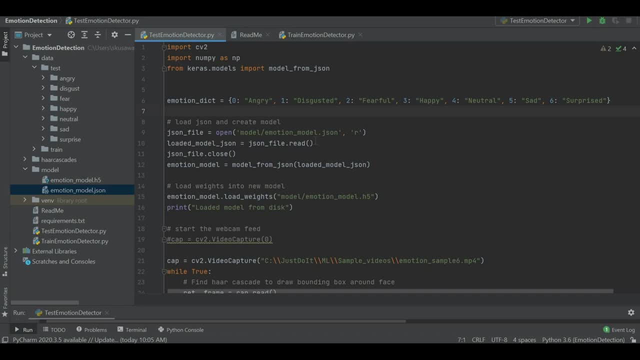 it is representing the angry emotion, okay, so i'll talk about it shortly. so now, here you can see that i'm loading our all trained emotion model structure. so whatever the model we have stored in this json file, i'm loading back and storing into the one instance. named it as: 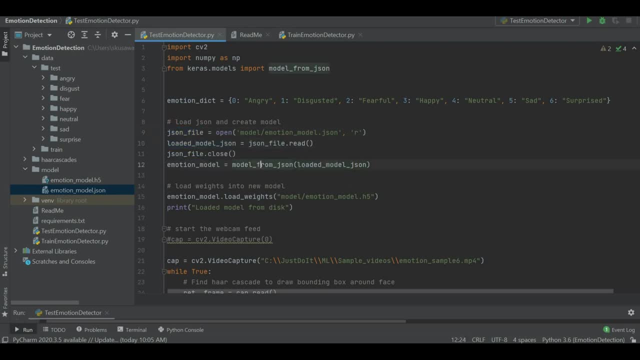 a loaded model json, okay, and after that i'm going to make use of model from json to convert that, whatever the json we have loaded into the model, okay, so here i'm creating the emotion model and once my model is created i'm going to apply all the weights or the learnings we have just stored. 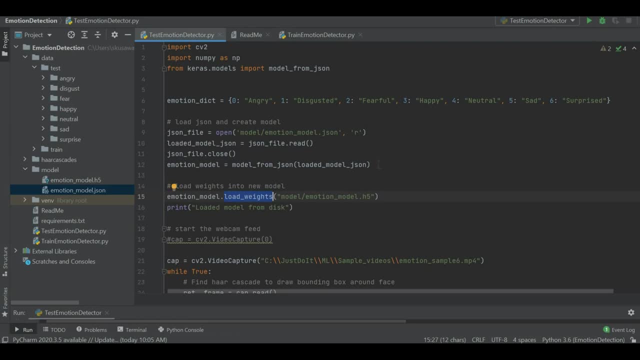 in this emotion modelh5 file. okay, so in this step, in short, we are just creating the all convocational neural networks which we have stored in the json file. we are creating back here with the help of model from json, and after that, whatever the model we have created, we are just applying. 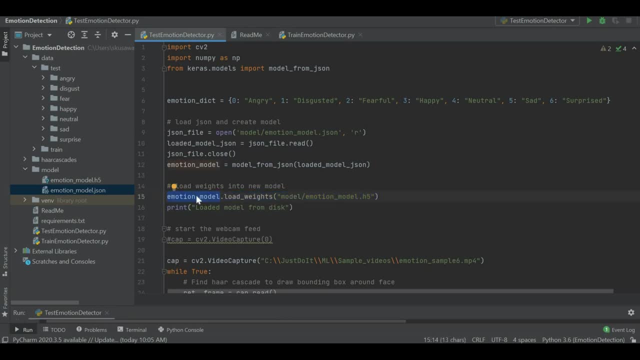 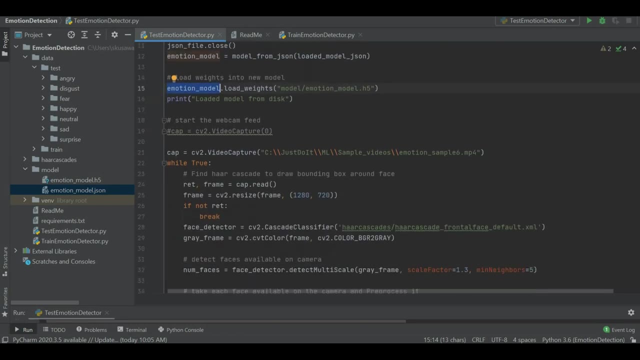 the loads or the learnings which we have made while our training. now our emotion model is loaded and ready to do the prediction. now we have to think about how we can read the input. so here you can see that i am making use of opencv. okay, so here i have commented the two lines of code. so 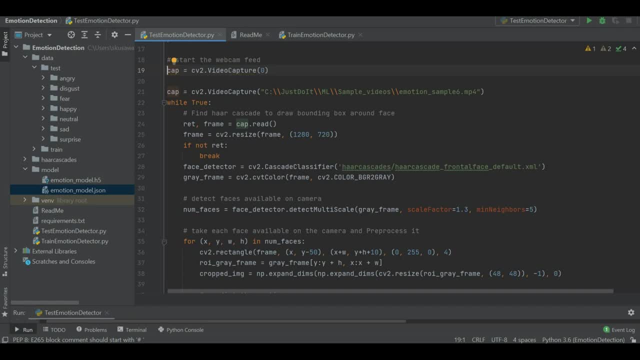 if you just uncomment this line of code, then it will access the all the inputs from your laptop's camera. okay, so as of now i'm just going to demonstrate you on the video, so i'm just going to comment it. if you want to check live from your laptop's camera, then you have to just uncomment. 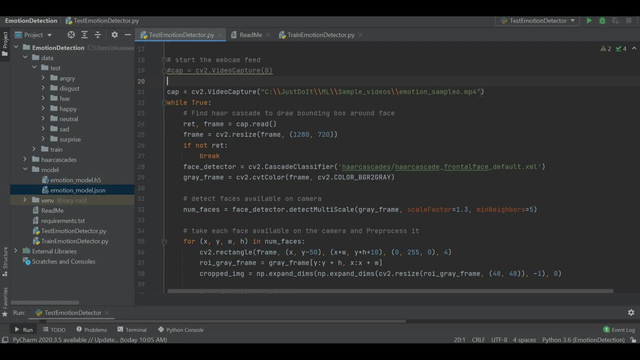 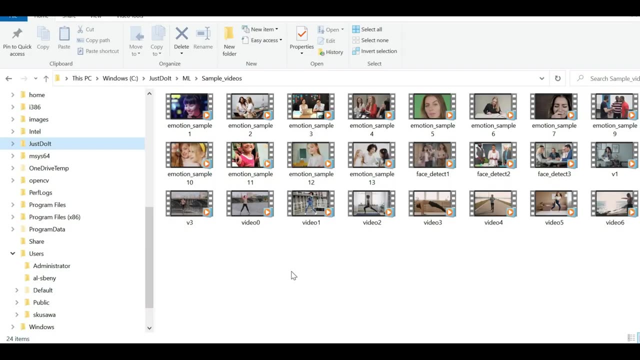 this line and comment the second one. okay, so now let's pass the one path of a video. so i'm having a couple of sample videos inside of my folder, so let me just quickly show you. okay, so here you can see that i'm having a plenty of sample videos, so i'm just going to 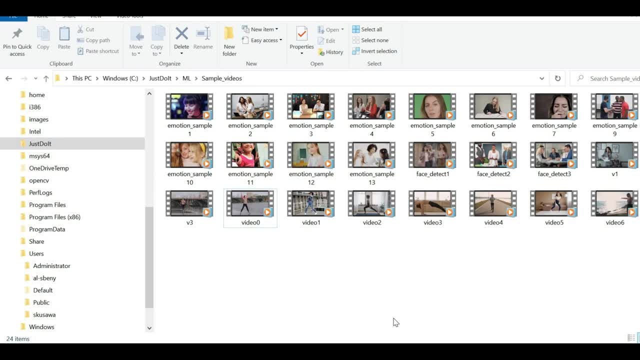 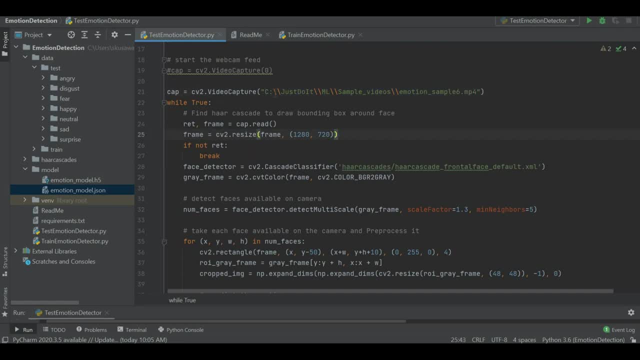 random videos from here and i'll show you how this emotion detection works. okay, so let's come back to our pycharm. so here we are, so i'm just passing the path of particular video. okay, so i have provided here double slash to just avoid any invalid characters, so it is a better practice to 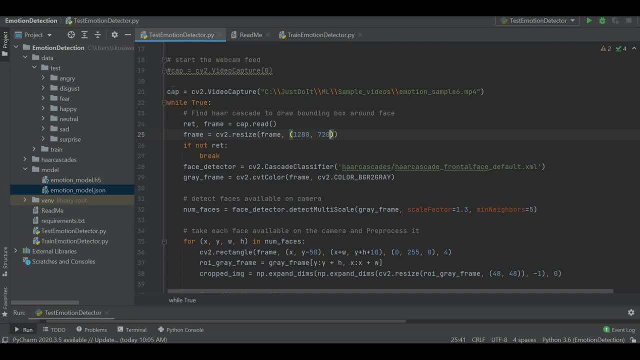 always follow that, and after that, whatever the frames, i am reading from this video, on that frame i am going to apply our model. okay, but before that we have to do some kind of pre-processing. so i am just resizing our all images to one: two, eight, three, four, five, six, seven, eight, seven, eight. 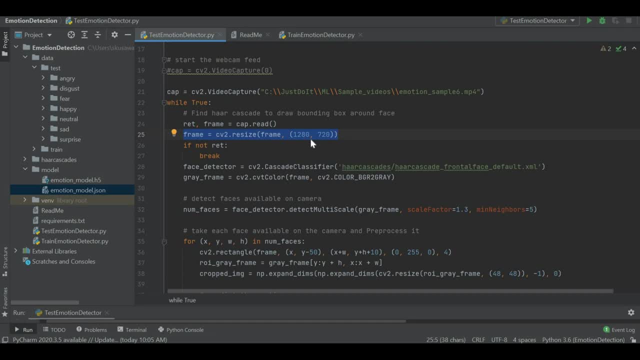 zero by seven to zero size, so it can fit well on my laptop screen. and here is an important thing, that. so, before uh, doing the emotion detection on the face, first of all we have to detect the face inside of our video or live stream. okay, so here i am going to make use of hard cascade classifier. 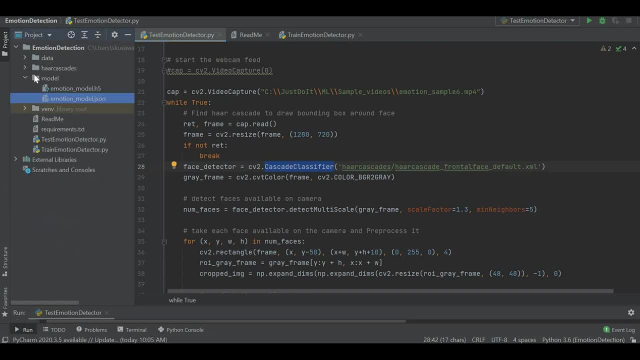 okay, so i have just created one folder inside of my project. so here you can see that i have created one hard cascade folder and i have plus this xml configuration of this hard cascade front face defaultxml file. okay, so, with the help of this configuration, we will be able to detect the. 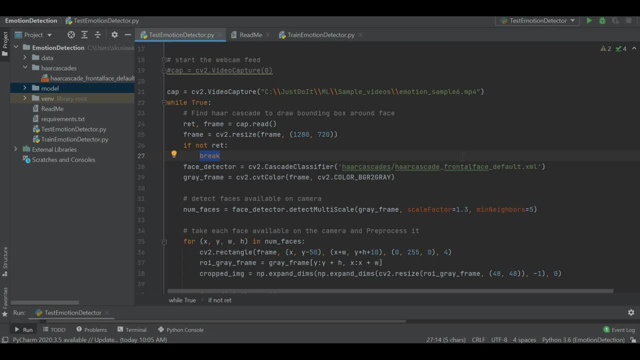 face inside of our video and then, whatever the face we are getting, that face we are going to pass to our emotion detection model so we can detect the emotion from this face. okay, so this is a two-step process. we can say: first we'll detect the face, crop it and we'll pass it to. 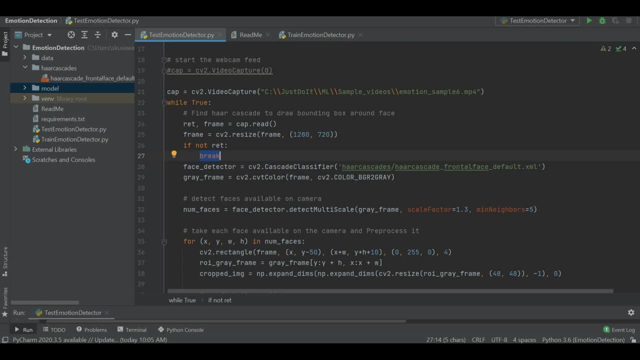 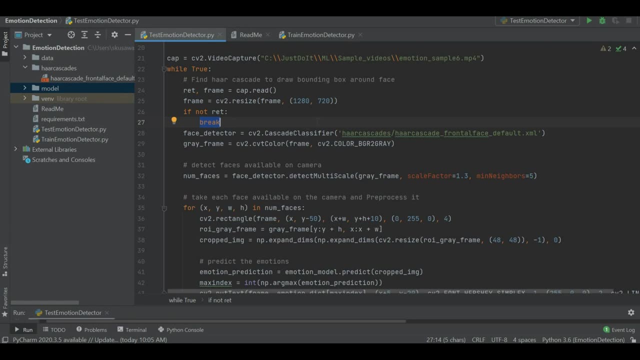 the emotion detection model, and emotion detection model will detect the emotion from that. okay, so i'll provide this actually hard cascade folder and the frontal face configuration for it on the github repository. so here we are making use of a hard cascade classifier and detecting the faces. so, whatever the result we got. so inside of that, 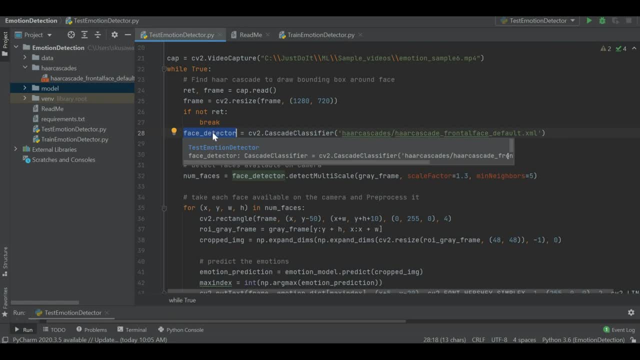 result: there would be, might multiple faces inside of that, because on video it might that four or five faces or two faces are there. so it has all details of all faces inside of this face detector. so from this face detector we are going to detect the all the faces and we are going to collect the 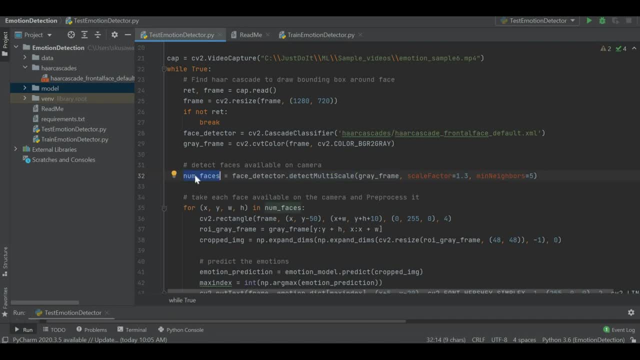 all number of faces available inside of that detected faces. okay, and i skipped this line. so here you can see that here what we are doing, we are just: whatever the image we are reading, we are converting into the grayscale. okay, because whatever the our model is trained, is trained on the grayscale images, so it will be able to identify the emotion. 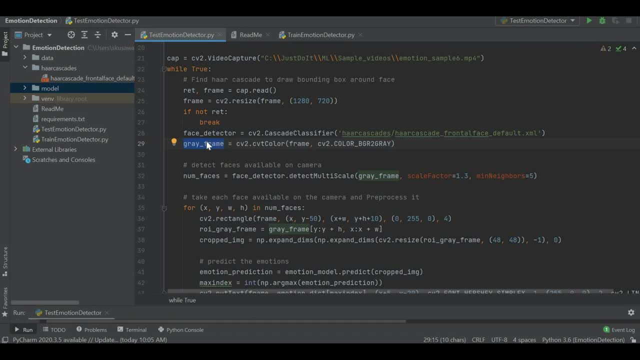 better on the grayscale image only if you pass the rgb image it might possible that it will give a miscellaneous result. so what we are doing, we are converting our image into the grayscale so we can crop the only face area on that gray image and pass it to our emotion detection model. 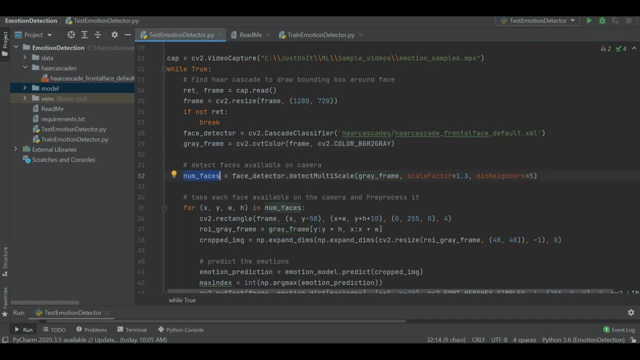 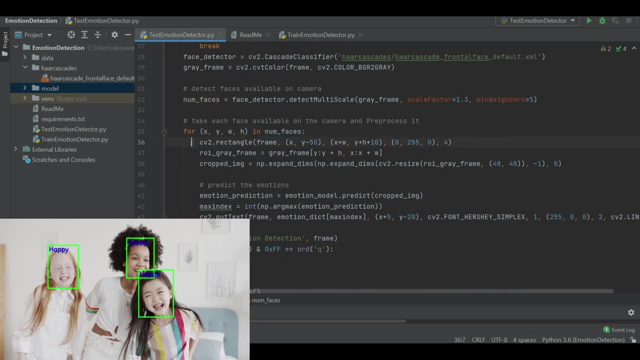 so, coming back to here, we are detecting the each faces and from this each faces i am going to access the each face: x, y and width and height location. okay, so it means that it will provide the position of the each face inside of that particular video stream or the live stream, so you can see that with 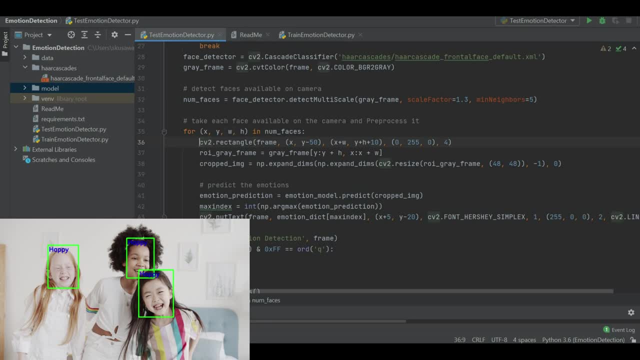 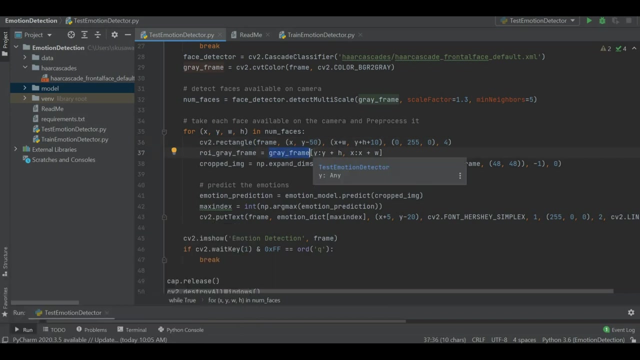 the help of this x- y and width and height position, here i am drawing the rectangle. okay, so this x- y position is a starting corner and width and height will help us to draw the rectangle around the each. so what i am doing? from this grayscale converted image, i am accessing or cropping the region of our 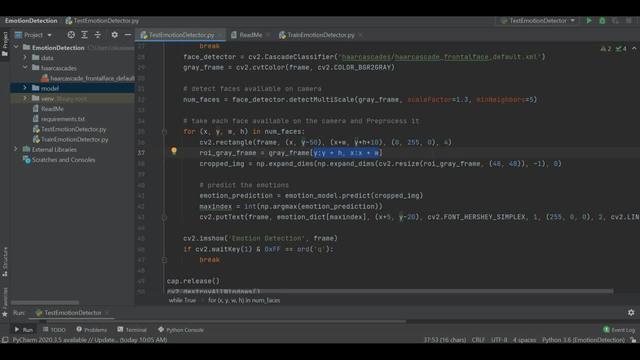 interest. so it means that whatever the full screen image we have or video we have from that, whatever the face images we are finding, i am cropping this, all the face images, and storing into the roi gray frame image. okay, so i am doing it for the each face which is detected with the help of this face. 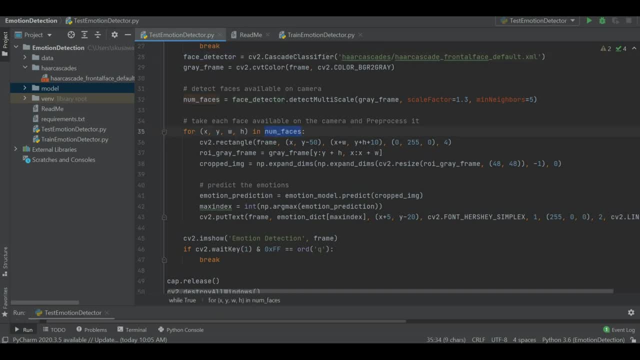 detector. so from face detector we are fetching the each face, we are accessing the x, y and width, height, and after that we are drawing the rectangle on the screen on each image, and, whatever the size we are getting, we are cropping the each face and storing into the one gray frame. okay, so after 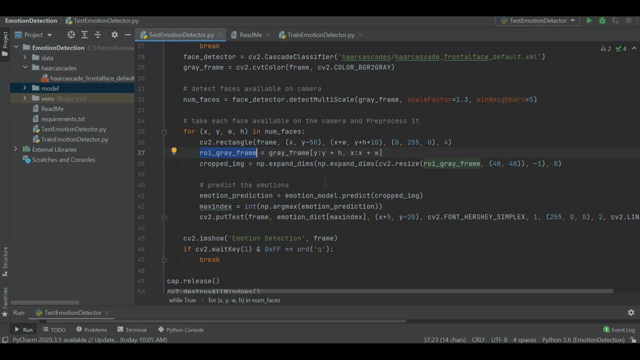 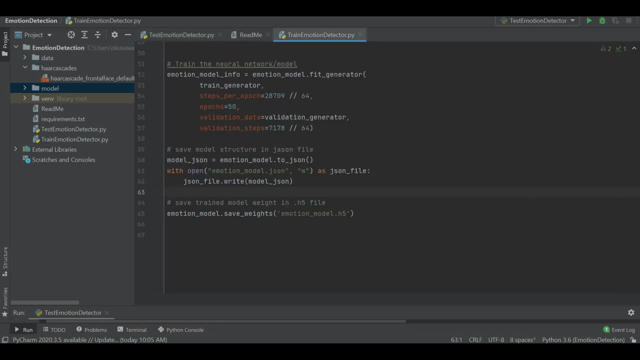 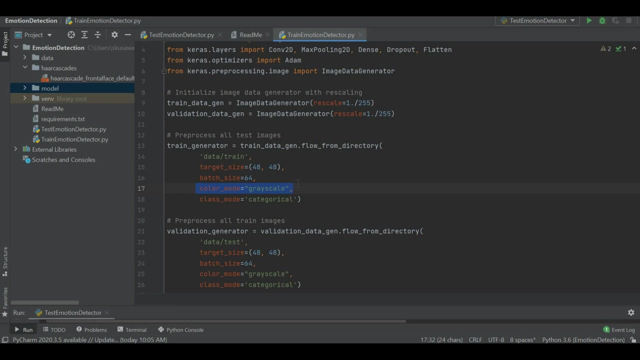 the cropping, the frame. we need to resize or pre-process our particular each face image before passing it to our emotion detection model, because whatever the our emotion detection model trained, so you can see that it is trained on the size of 48 by 48 and with a grayscale color, so similar kind. 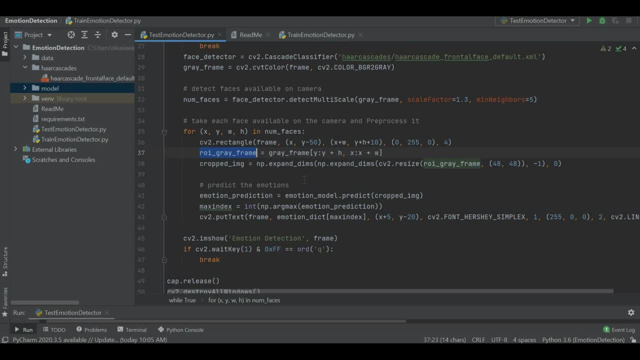 of processing we have to apply while testing it. so here you can see that, while detecting what i am doing, whatever the image, face image i am getting, so that face image i am converting into the 48 by 48 pixel size, okay. so here you can see that i am resizing it and expanding its dimension and 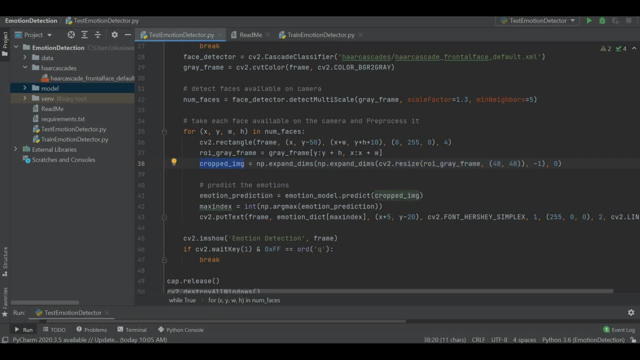 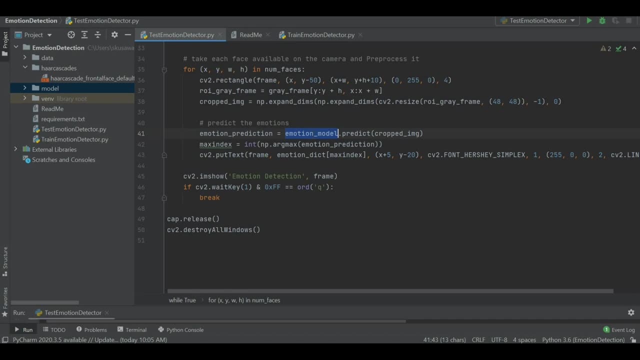 whatever the crop image i am getting, this cropped image i am going to pass to our emotion detection model for the prediction purpose. so here you can see that this is our emotion detection model and i am going to do the prediction. so, whatever the pre-processed faces we got on our video or live. 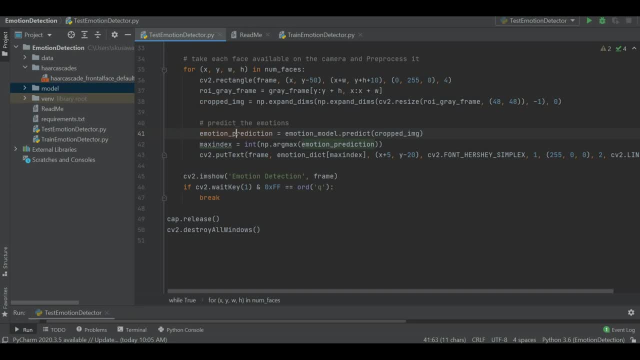 stream i am going to pass to this model and it will provide me the emotion prediction result. okay, so in outcome, we'll get the list of the all the emotions and the percentage of confidence. our model is feeling about these, each images. so in output, in short, what we'll do, we'll get. 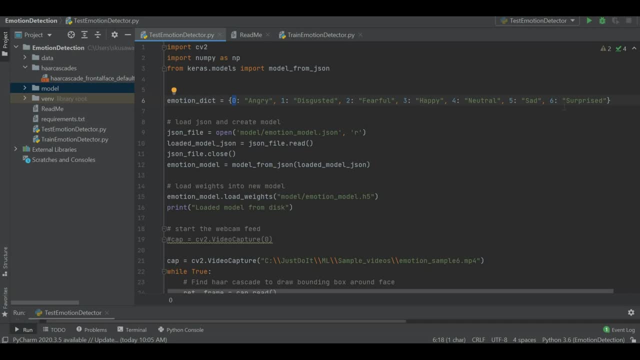 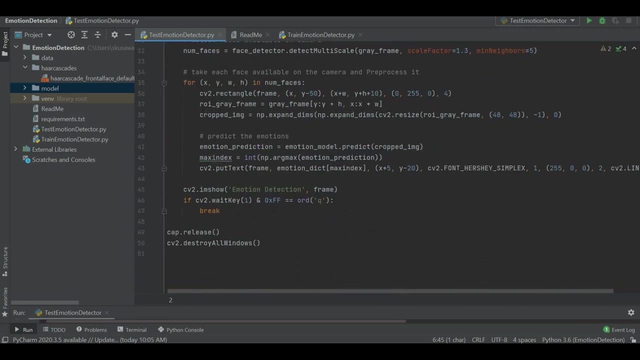 the list of these all emotions like 0, 1, 2, 3, 4, 5, 6, and how much percentage it feels like it is a zero emotion or the angry emotion, or how much percentage it feels like it is a two emotion, that is, a fearful emotion. okay, so this kind of list will get and the percentage of each emotion. 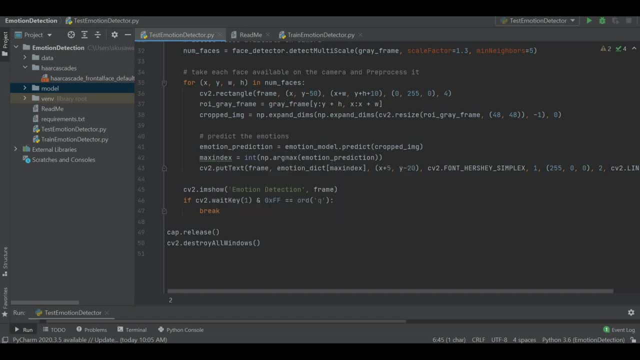 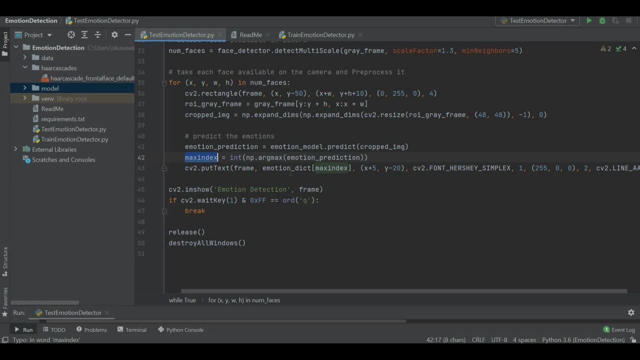 confidence will get and from that what we are doing, we are getting the max emotion confidence and it will provide us an index, and that index would be nothing but we are going to put on our emotion detection dictionary, which i have just created over here on top. okay, so i'll just pass. 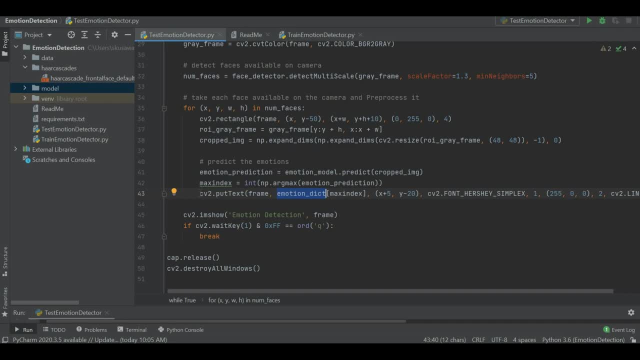 here the index of the emotion, and that emotion will be printed on our screen. okay, so you can see that we are using open cv put text and whatever our original image. here i am providing the predicted emotion and this is the positioning of that particular text and font and all, okay. so 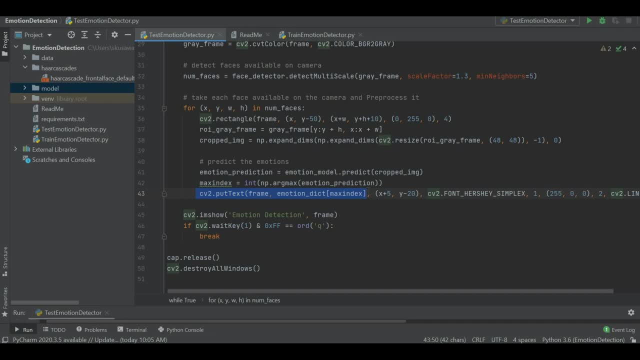 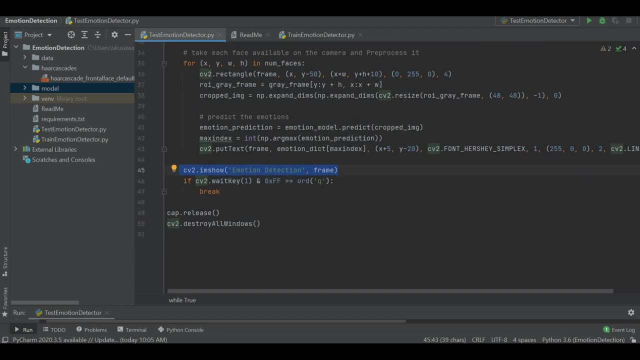 in short, we are just putting the what emotion we have predicted just above to the rectangle box of our each face, and here we are just displaying our output image with whatever the faces we identified and what is the emotion we have identified. and here we are doing the release of all resources we have allocated. now let me just quickly go and 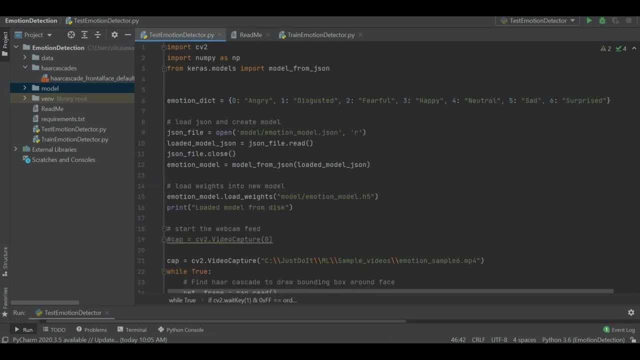 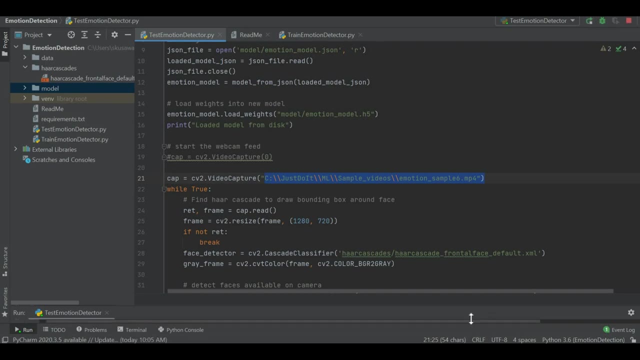 run this code and show you that how this emotion detection works. okay, so here you can see that this is our sample video on which we are going to check. so let me just try to run it so you can see that on the console it is running. so let's wait while our model gets loaded and 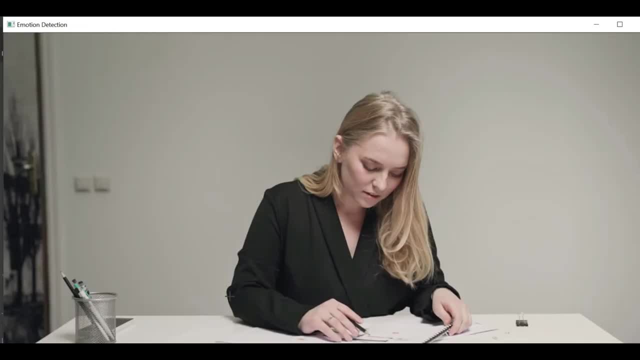 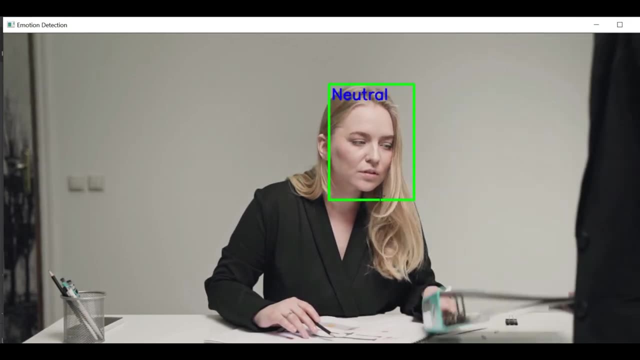 it start applying on the video stream. okay, okay, so now you can see that our video is open. so we are going to run it, and we are going to run it, and we are going to run it and you can see that it is doing the emotion detection on this particular face. so, on our video. 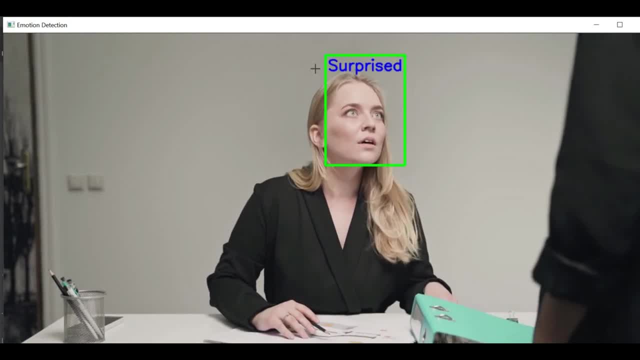 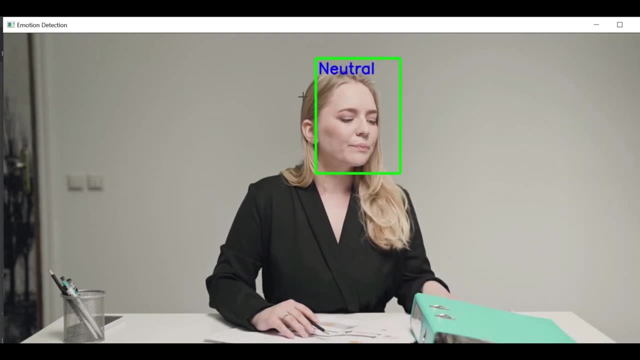 it first detected the face inside of frame and after that it drawn the rectangle and then it passed this face to our emotion detection model and our emotion detection model is now detecting the emotion and printing over here so you can see that neutral emotion and as we go ahead you will. 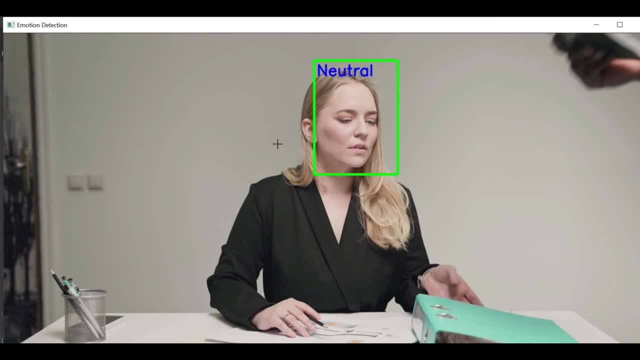 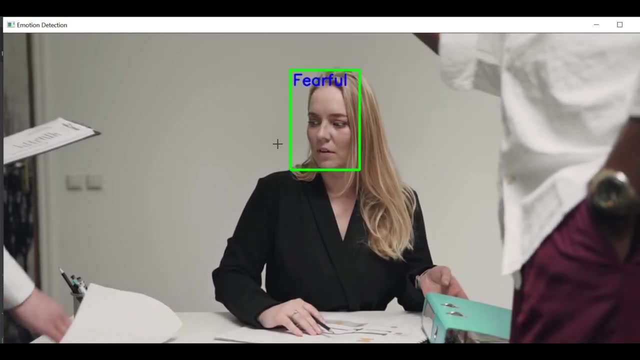 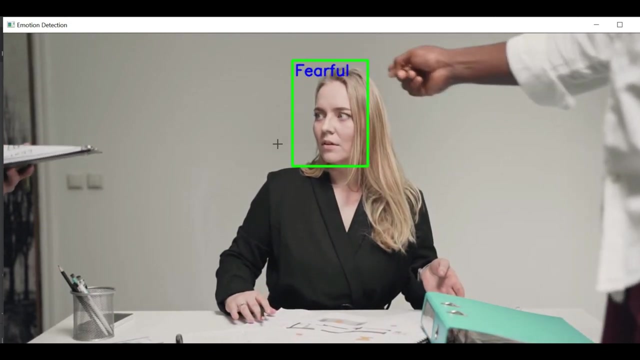 see the change in the emotion as the expression on the face of this woman get changed. okay, so you can see that now it's going to the fearful, neutral, surprised, and as the facial expression changes, our emotion detection model is smart enough to identify the emotion based on its learning made with the 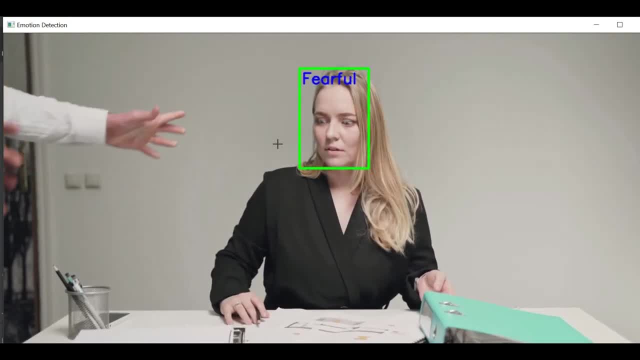 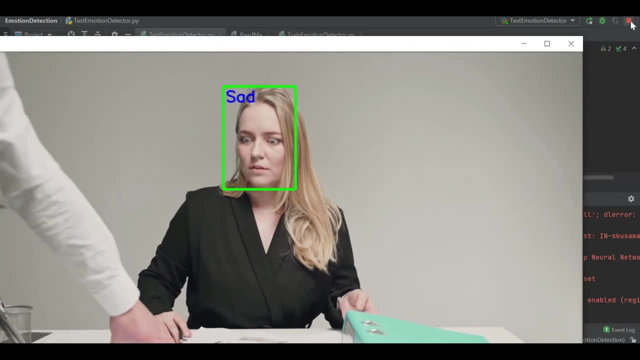 help of far 2013 data set. okay, so now let's go and try with some other video and let's see that what kind of results we are getting. so i'm just going to put this video aside, let me just close this and let me just go inside of our code and provide some other input. okay, so let me just 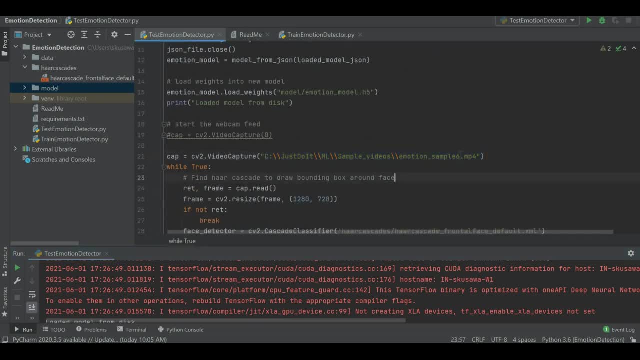 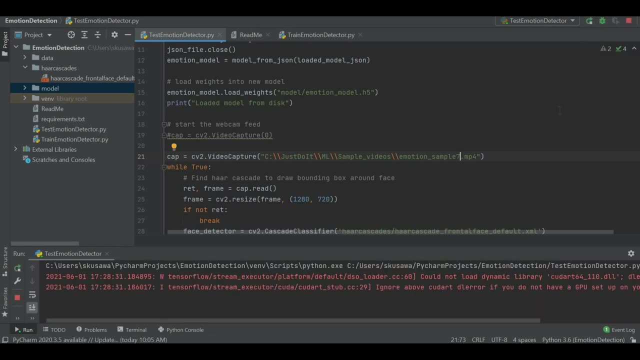 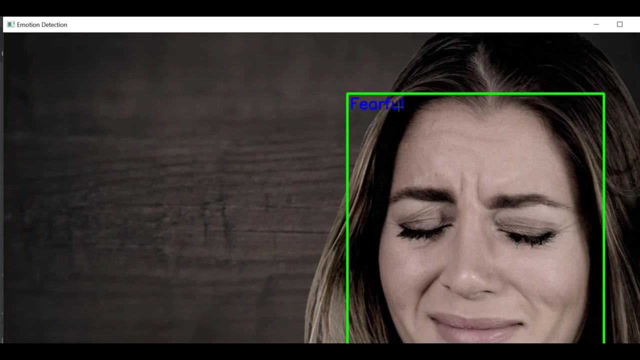 run the code size bit and here, okay. so here we are going to provide some other samples, like a emotion sample seven. okay, and let me just try to run it. okay. so here it is. so here you can see that we are seeing the face and we are getting the emotion like a fearful, disgusted. so as the facial 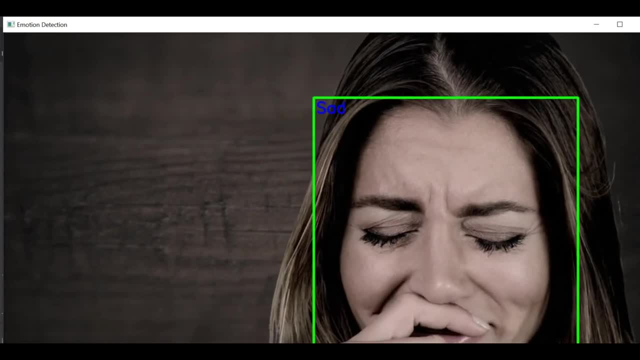 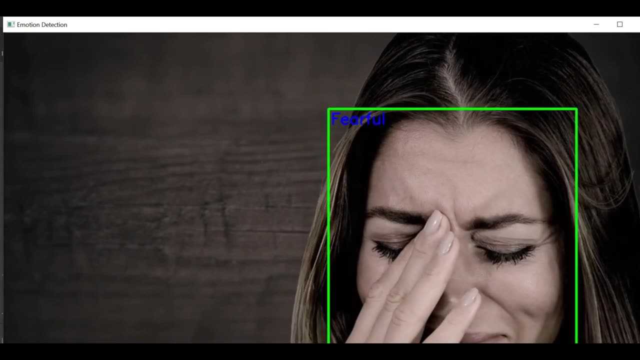 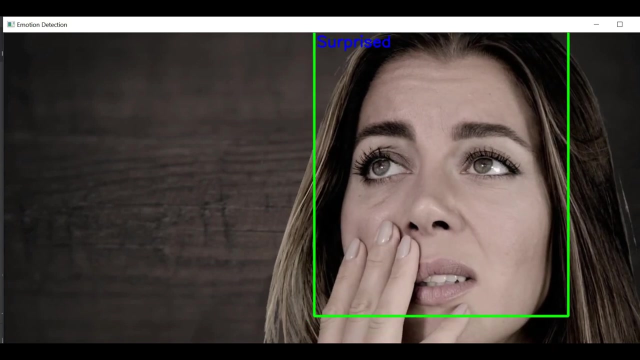 expressions are changing the automatically. our emotion detection model is smart enough to identify the emotion. okay, so you can keep observing that. now a woman is in the sad or fearful situation, and as soon as it started showing the happy emotions on face, you can see that our emotion. 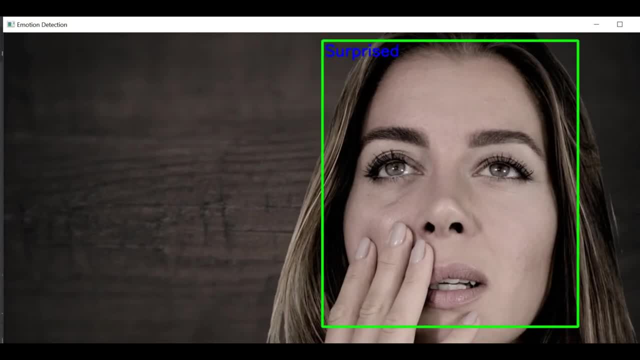 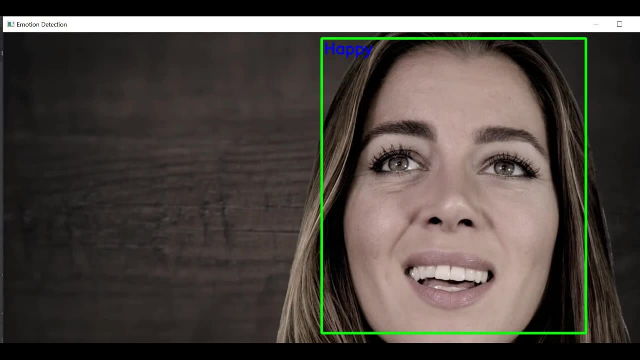 detection model will be easily able to identify it. okay, so you can see that, as keep going, the emotions are changing. as it starts smiling, you can see that our model is detecting that it is a happy emotion. okay, so now i guess our model is working fine and it is giving a good 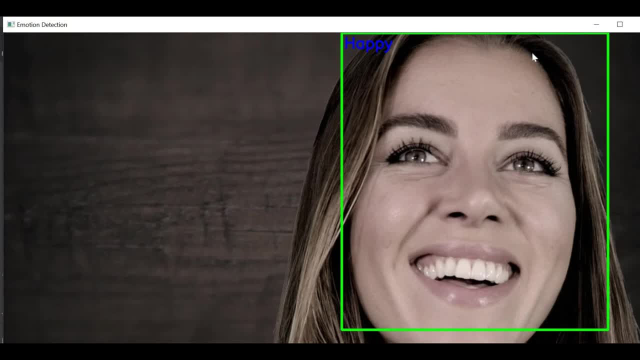 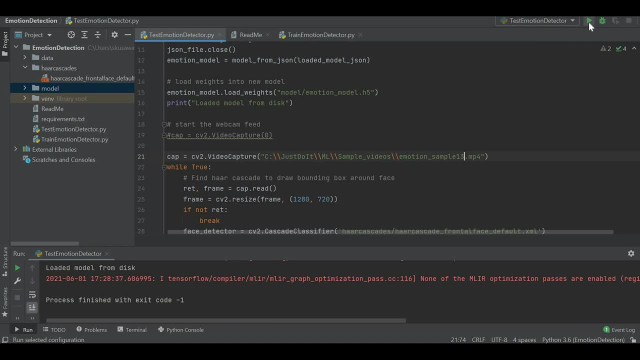 result: okay, so let me just try with one another video. so let me just stop this one and go back to our code and let me just try with something, uh, other sample. okay, let me just try to run now and let's see that how well it works on the multiple faces at a time. okay, so let's wait. our model is. 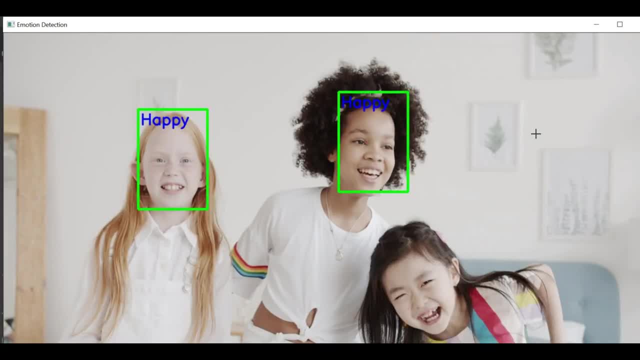 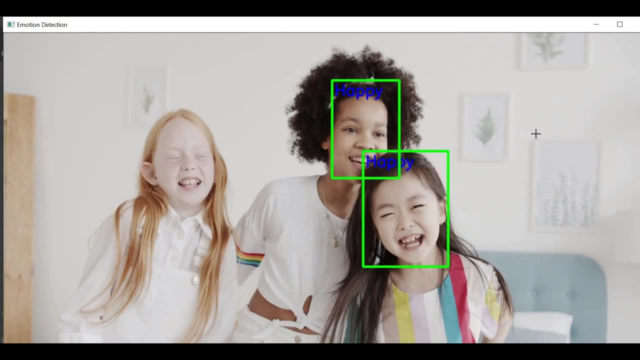 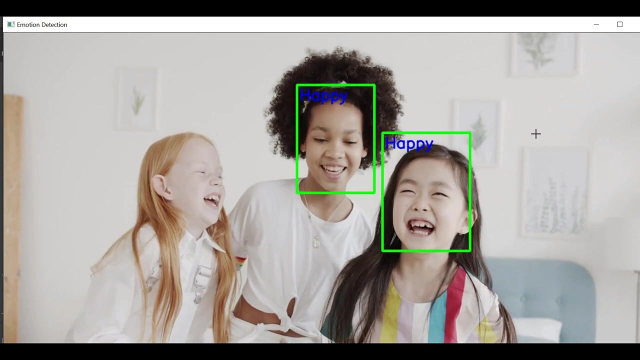 getting loaded and, yes, now model is ready. okay, so now here, you can see that we have a couple of kids on the screen and you can see that it is detecting the emotions very well. okay, so even it is a multiple faces, it is doing a very pretty well job. so, as of now, i'm just 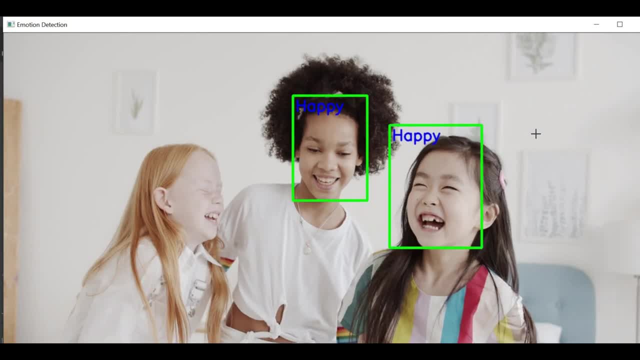 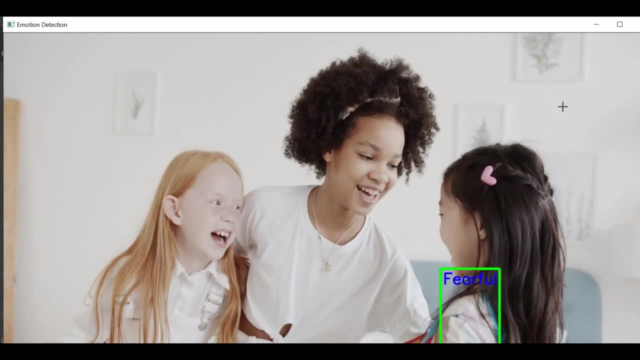 running it on a cpu. if you are using a good system, then might it will work a bit better because it will process the frame faster and it will provide us the better result. okay, so you can see that when the people are, face is not completely visible or the complete all the face landmarks. 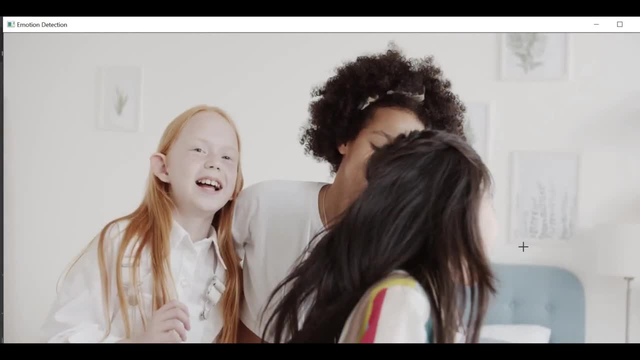 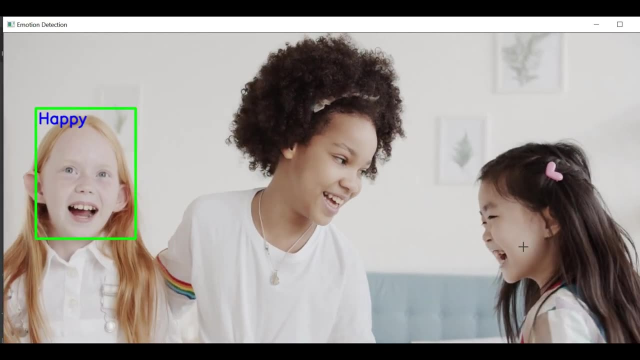 are not visible on the screen, in that case this face detection model is not working well. but when the actual face is not visible, then the face detection model is not working well. okay, so now you can see that when the face or complete face is visible on the screen from the frontal side in 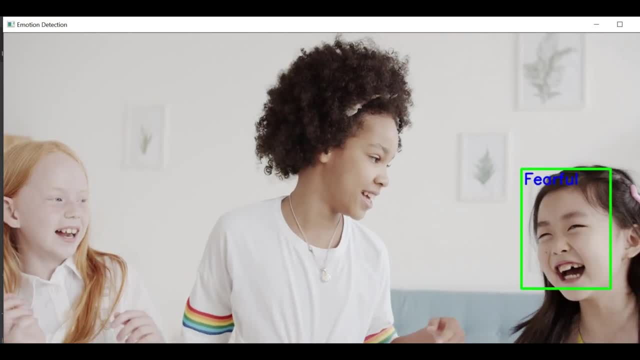 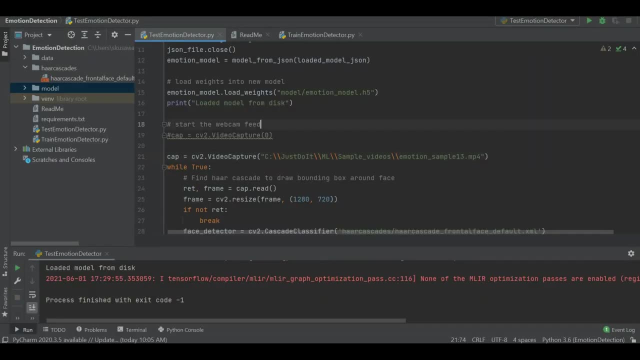 that case, it is working fine. okay, so why it is happening? because whatever the face detection algorithm we are using, okay. so let me just close and show you quickly. so, whatever the face detection algorithm we are using, that is the hard cascade. okay, so it is a frontal face. 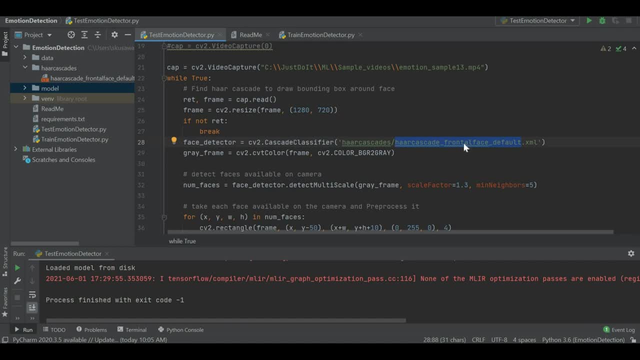 so it is only able to detect the faces when these faces are in the front direction and all the landmarks are visible. so if you want to get the more accuracy or want to identify the faces in a more, better way, then you can go for the other algorithms, which gives a better. 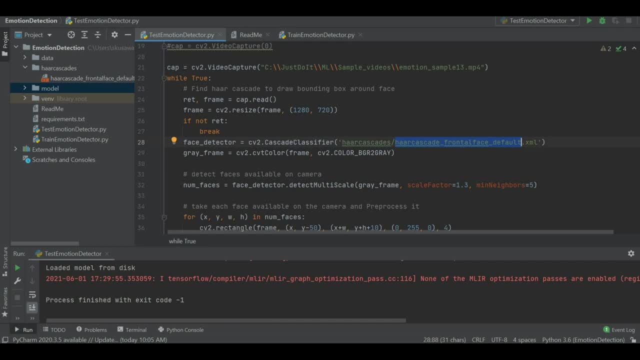 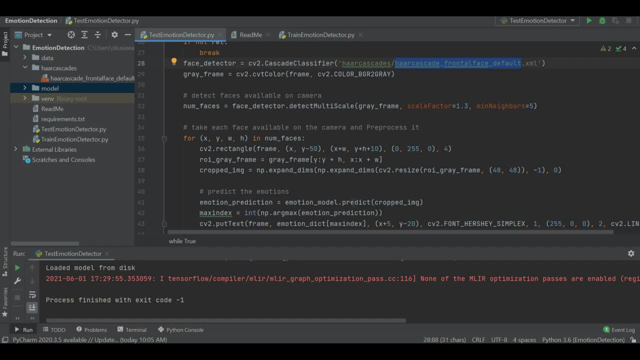 accuracy or better, face detection, and after that you can apply our emotion detection model, then in that case it will be able to detect emotions. even the 75 percent or 80 percent frontal face is visible on our screen or live stream. okay, so that you can take it as a homework.